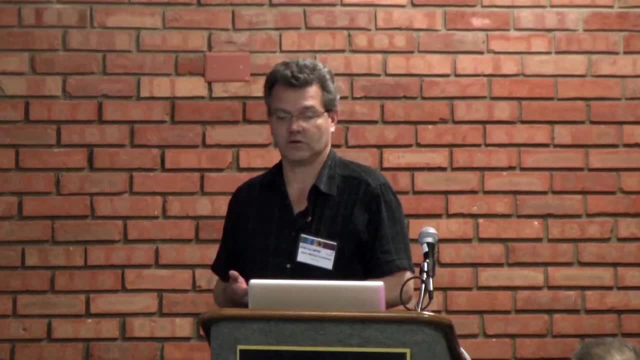 There's a huge number of increases in cores. There's a lot of architectural diversity. So there's CPUs, GPUs, APUs, which combine both CPU and GPU onto the same chip. There's ManyCore, the Xeon Phi or the Intel Mic, which you may have heard of. They're the same thing, just two different names. 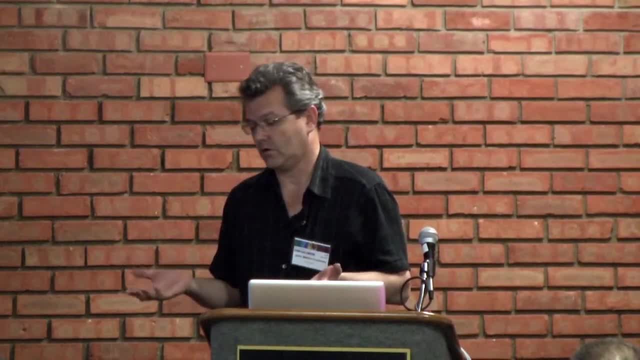 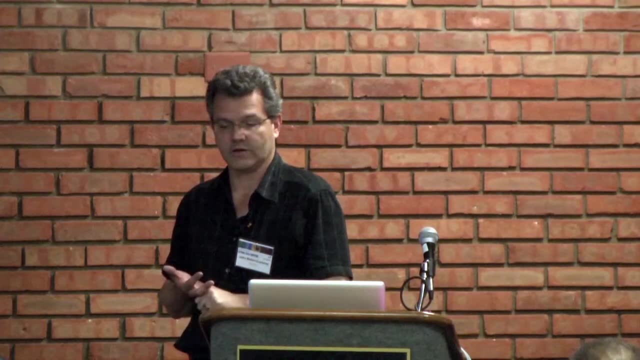 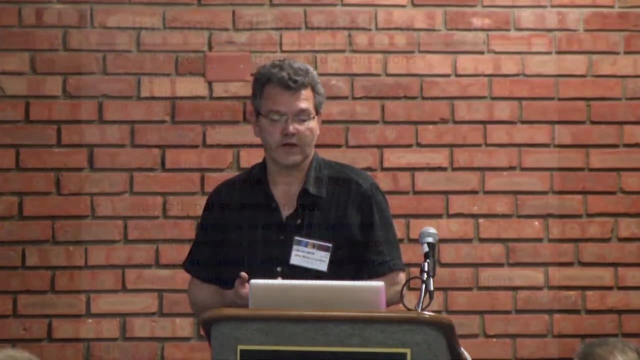 And also the parallel systems. they're increasing in scale. So the systems like Sequoia and Mira really make it daunting for application developers to scale all the way out, And also it poses a huge challenge for tools, And so on the application side, you may be working on a new application or you may be just working to augment the capabilities. 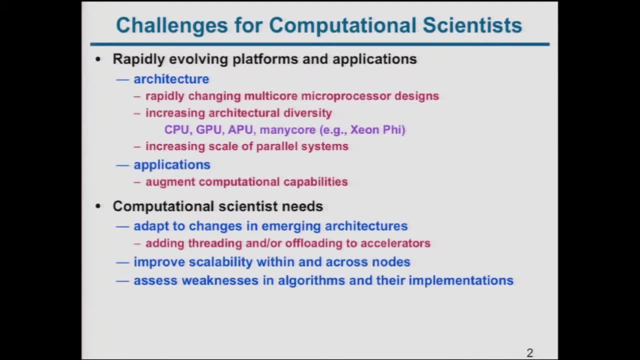 of an established body of code, like the Flash code that we heard about earlier, But, in any case, not only are the architectures evolving, but your applications are evolving too, And so what you need to be able to do is to adapt to the changes in the emerging architectures and be able to improve your scalability. 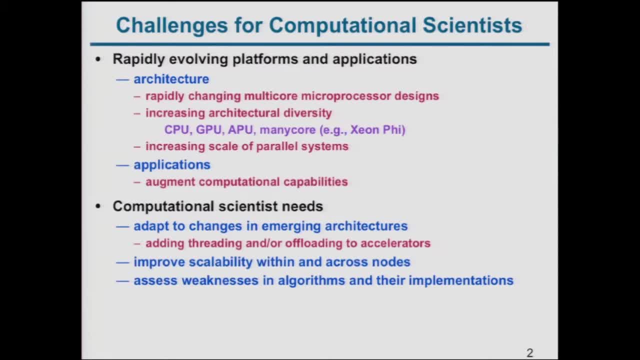 both to larger numbers of cores on the nodes, or take advantage of GPUs, or to improve your scaling onto these larger scale machines so you can tackle larger problems. And then you need to assess weaknesses in your algorithms and implementations and decide where you need to invest your effort if you're going to get the most out of your allocation on these systems. 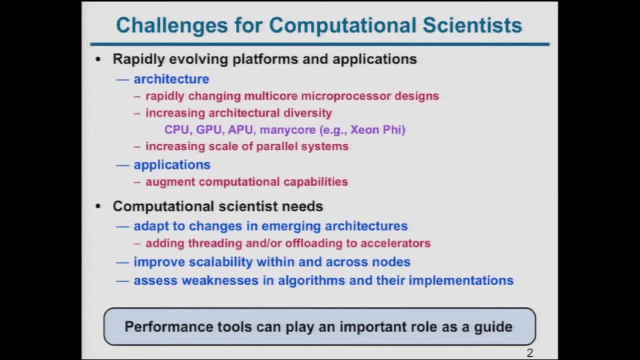 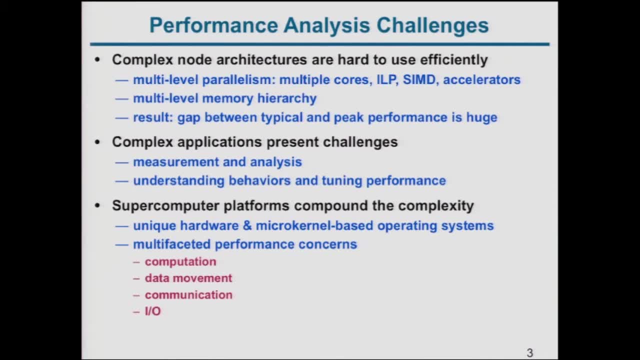 And so performance tools can really play an important role as a guide in deciding where and how to invest your effort And so on today's architectures, they're very hard to use efficiently, So we have complex node architectures with multi-level parallelism. You've got multiple cores. 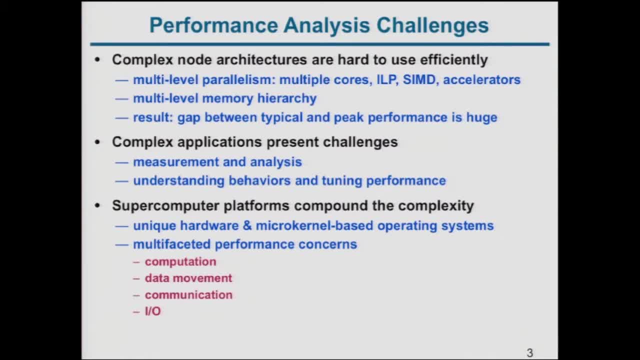 You've got multiple nodes, instruction level parallelism, short vector units on the Intel processors and on the Blue Gene Q. You've got accelerators like the Intel Mic and GPUs, a multi-level memory hierarchy, And so, as a result, the gap between what's the possible performance you can achieve and what you actually achieve is huge. 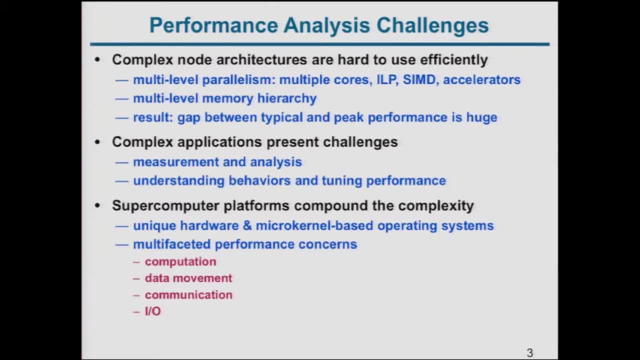 And so typical scientific codes might get, say, 5% of peak if they haven't been tuned- A well-tuned code- you might bring it up to 25% of peak with a lot of effort, And so there's a factor of 5 in there, and so that can make or break how well you succeed with your allocation and whether you get your science done. 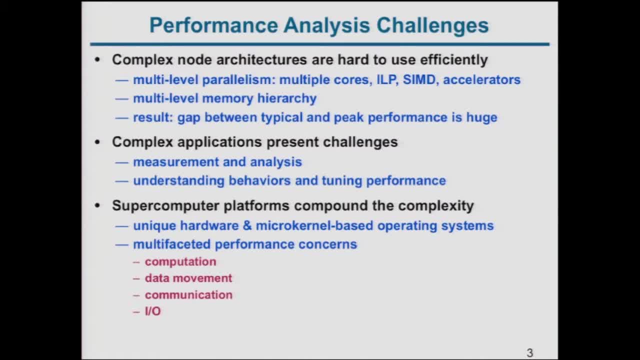 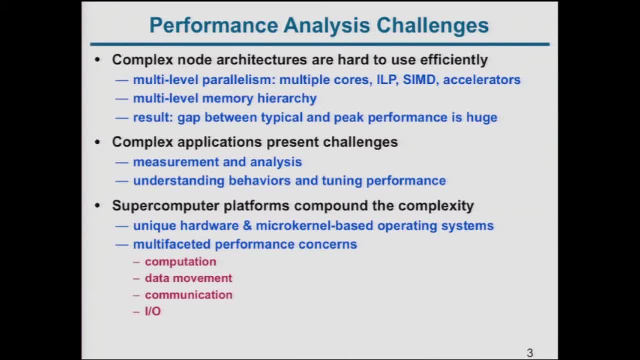 And so these are challenges for both measuring and analyzing your code and understanding their behavior so that you can tune their performance. And then, on systems like Mira and Titan, you're interested not just in the computation, but also in the data movement and the communication and the IO. 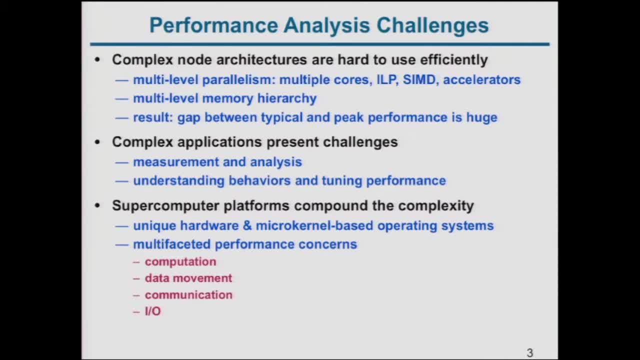 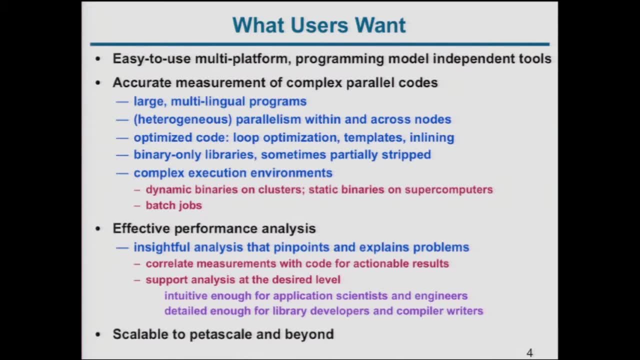 And so we have to be able to capture information about all of them. So what I would argue that you want are easy-to-use modules. Use multi-platform, machine-independent programming model, independent tools so that you can use them with MPI, Or there's trends nowadays to use Unified Parallel-C or Coray Fortran. 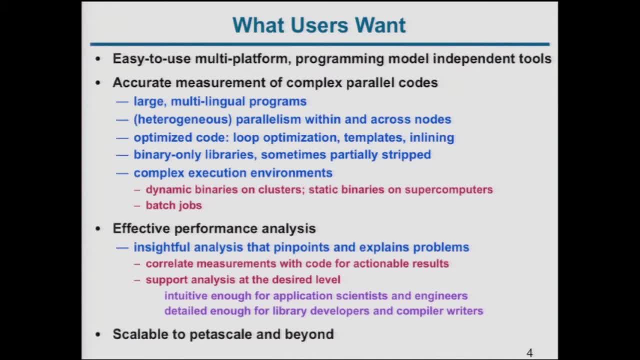 And so you'd like to be able to use the same tools regardless of what programming model you're using. You'd like to have accurate measurement of complex parallel codes, in that the codes may have a mixture of C++ and Fortran. You may have heterogeneous parallelism within and across nodes if you're using, say, GPUs and your CPUs. 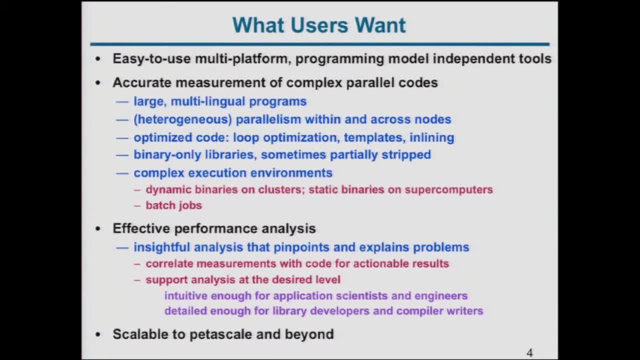 And the only code that it makes sense to actually measure the performance of is optimized code. Because if you turn on the optimizer and you get a factor of three- performance improvement- then it doesn't make any sense to turn off the optimizer and then measure the performance of your code. 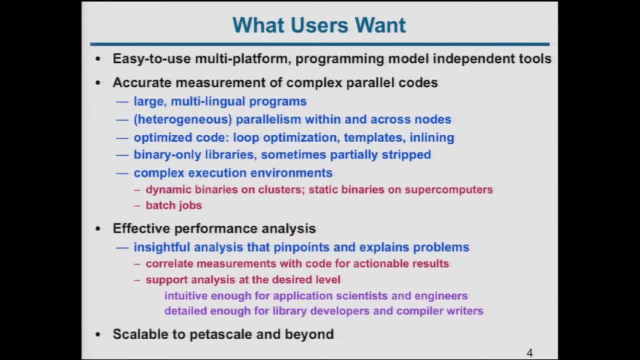 So what you want to be able to do is compile your code sort of flat out the way you'd like to run it on the system as a protocol, And then you want to go back to the production code and then measure its performance that way. 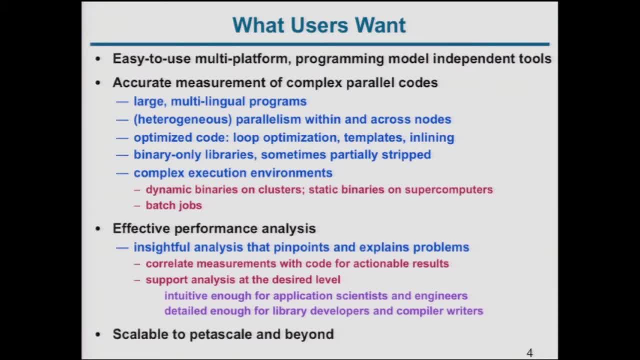 And then find out what's left that you actually have to pay attention to, because the compiler couldn't get it, And so you need to deal with the fact that some of the libraries are available only in binary form. Sometimes they're partially stripped, like the GPU code. 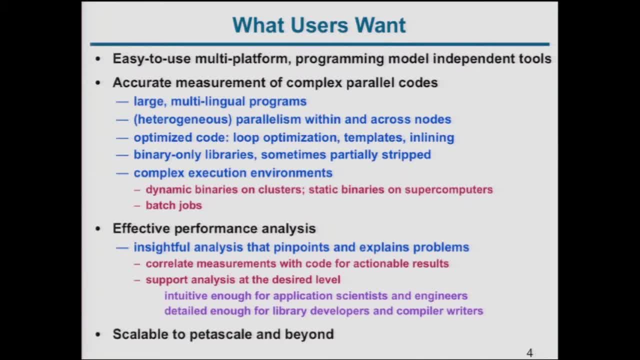 And you're looking for some tools that are going to be able to provide some insightful analysis and pinpoint and explain problems, And so you need to correlate any performance measurements with the code In order to figure out what you're going to do about it. 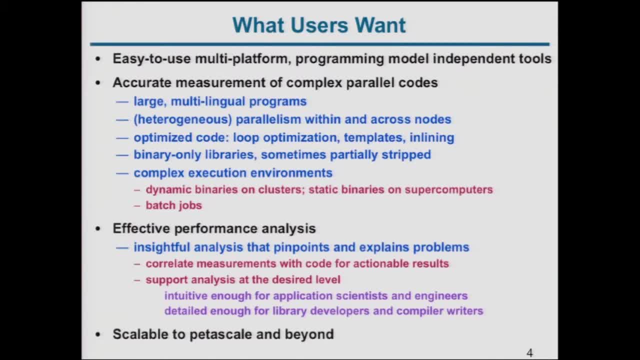 And so I would argue, often for scientific codes, that means taking the performance measurements and showing them at the loop level, Because the loop level is where you can make changes in scientific codes. And so we show things at the level of loops, procedures, call chains and several different views, as I'll get into in a few minutes. 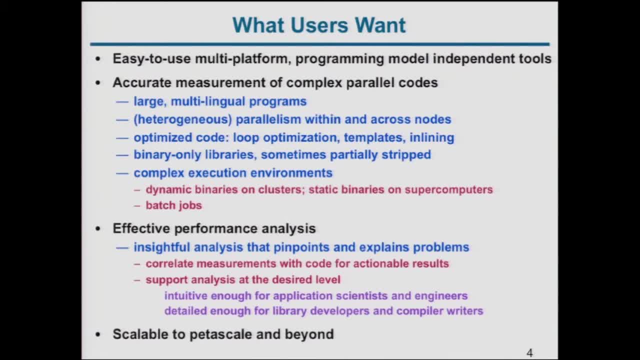 And then the tools have to scale to these large scale machines And, as Mike mentioned, we can collect for a fraction of processes rather than collecting for all, And that's one of the ways that we deal with scaling. So what our HPC Toolkit performance tools do. 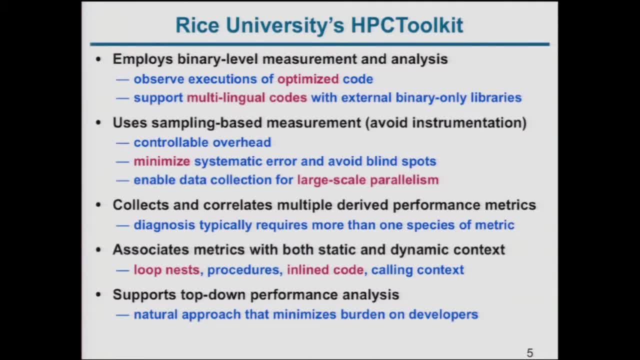 and I should make a point of saying that there's actually two sets of tools called HPC Toolkit. There's ours from Rice University, And then IBM also has something that they call HPC Toolkit, except that they have a space between HPC and Toolkit. 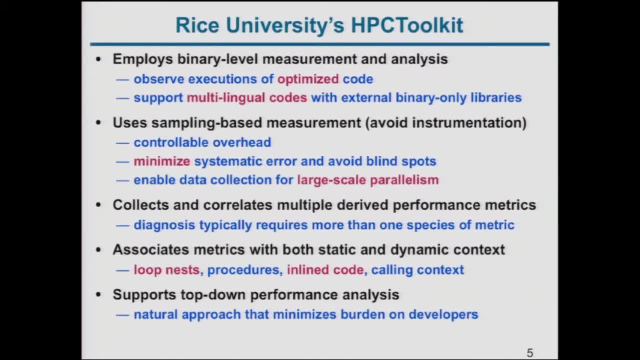 We both chose our names back in 2001.. We both, just like, searched the web and didn't find anybody that had the same name, And so, anyway, if you search the web now, you'll find that ours is the number one hit. 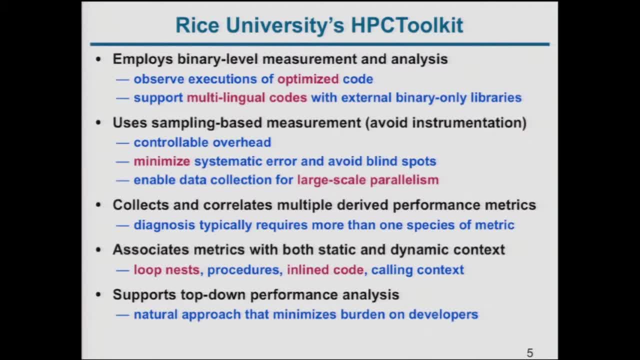 So we don't care what IBM calls their tool So, and ours is free, But not as free as you'd think, So we'll be talking to you about a support contract. So what our tool does is it employs binary level measurement and analysis. 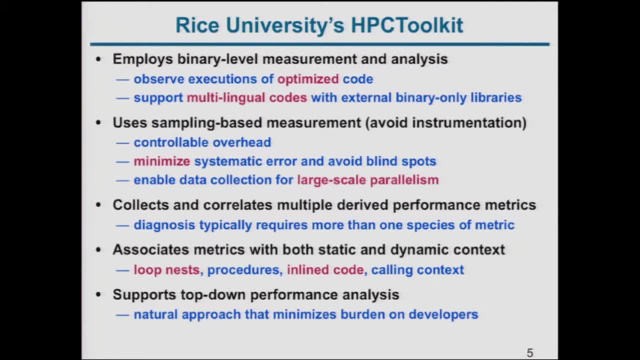 And so what you're doing is that you're observing executions of objects, You're optimizing code, And it supports multilingual codes with libraries that are available in binary only form. You use sampling based measurement, as the previous speaker said, And so with sampling you get controllable overhead because you can decide what your sampling frequency is. 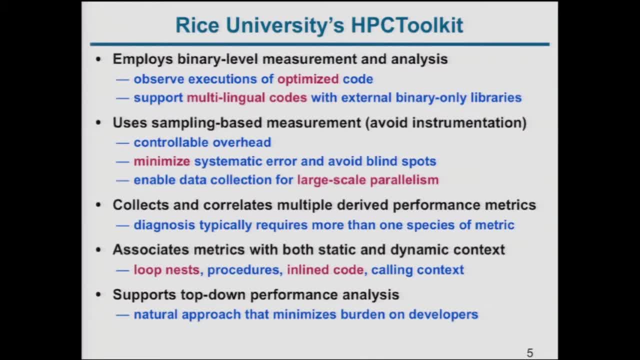 You can decide: I want to sample 1,000 times a second or 100 times a second, or I want to sample using hardware counters and say every 3 million instructions or every 2 million L2 cache misses, And so by dialing up the period you can reduce the sampling frequency and reduce your overhead. 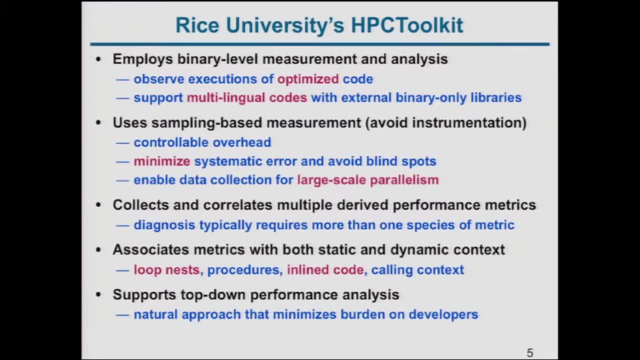 And so, since we work on multiple architectures, we haven't set any particular sampling rates, And if you have an application that's running for 10 seconds, you may want to sample it a lot more than an application that's going to run for 2 hours. 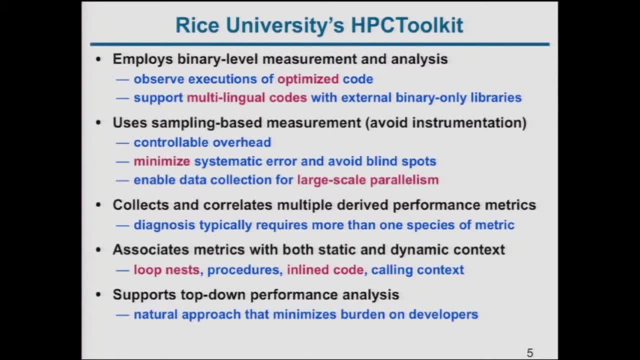 because, in order to make the kinds of judgments that you need when doing performance analysis, what you need is a useful number of samples, And so how you acquire that number of samples- whether it's with a low frequency or a high frequency- sort of depends on what your run time is. 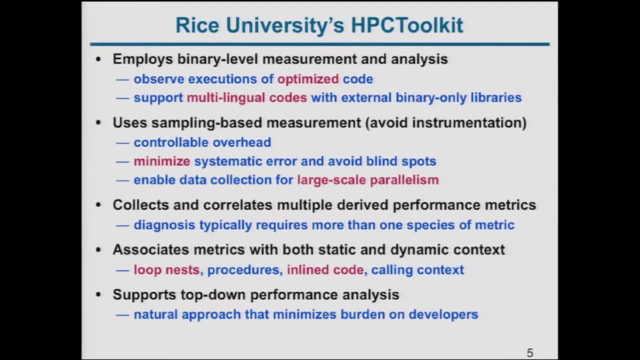 So we leave that as a knob that you can turn, And if you find that your program is slowing down too much when sampling with a particular period, then you can just increase the period as you see fit. So it's got controllable overhead. 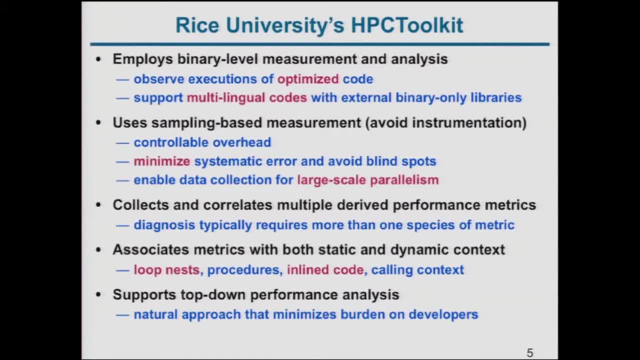 It minimizes systematic error by avoiding blanks. So you see the time that's spent not only in your application program, but in all the things in libc, all of the math libraries you use, whatever. And in order to collect performance information, you can find out where you're spending your time just by collecting something like wall clock time. 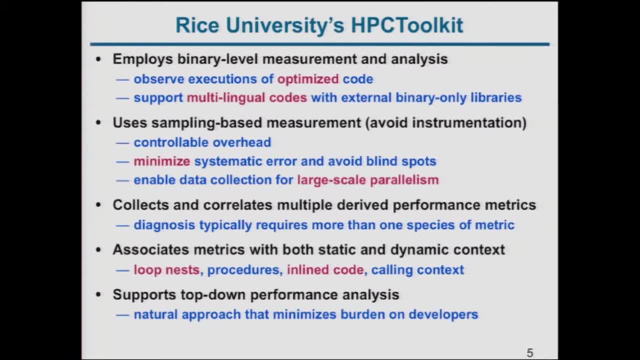 But often to get into the details of well, am I spending my time? well, you need to use hardware performance counters, And so that means collecting multiple metrics, not just one metric. like time, Often, you'll need to collect floating point operations. 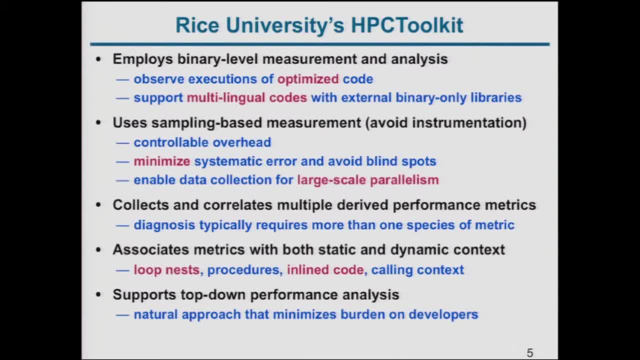 or L2, misses or cycles or things like that, and look at the ratios of these things to decide how well your application is doing, Although I'll show you you can do a lot with just time. And then we associate these metrics with both static and dynamic context. 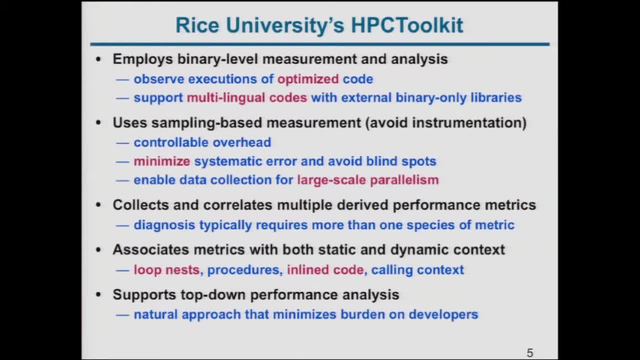 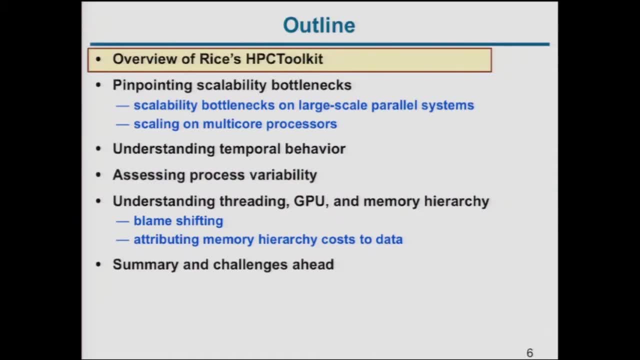 And so loop nests are a unique thing to our tool. We can also associate costs with inline code as well, and then support top-down performance analysis. So let me give you a brief overview. So this is not going to be a manual for how to use the tool. 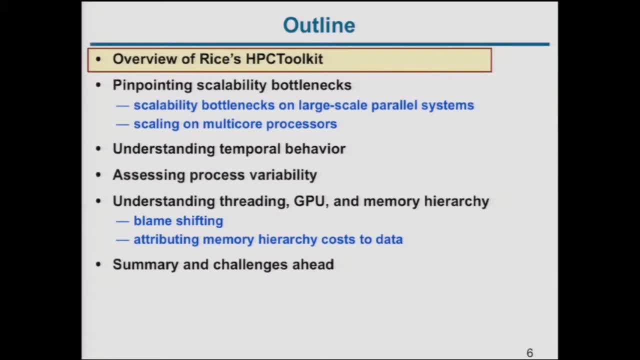 This will give you a flavor for how to use it. There's some more detailed instructions online in our manual and also at the ALCF website, And I'll be around this evening if anybody's interested in giving it a try. So this is going to be sort of a hand-waving how it all works. 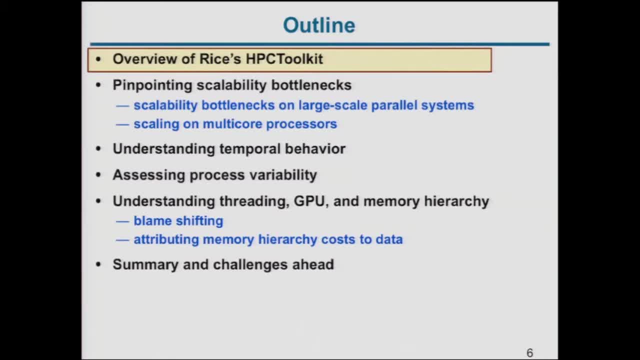 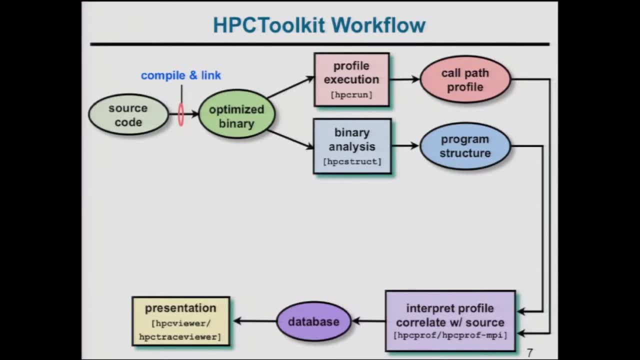 and I'll do a couple of live demos, if I can squeeze them in, and tell you some of the things that you can do with our toolkit. So this is the workflow overall. So you start out with your source code and you compile and link it the way you normally do. 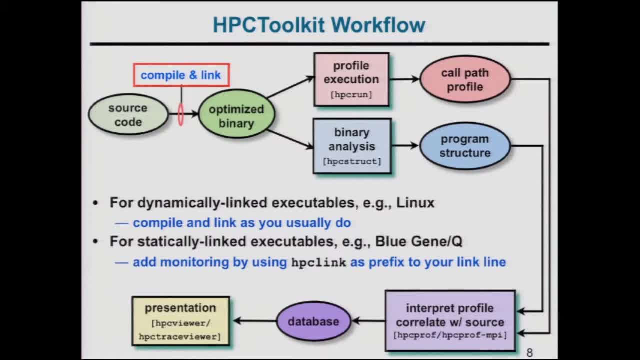 And so for dynamically linked executables, as you would use on a Linux cluster, then that's all there is to it. You just use your normal make files and then you launch your application with a launcher script that we provide Now for statically linked executables. 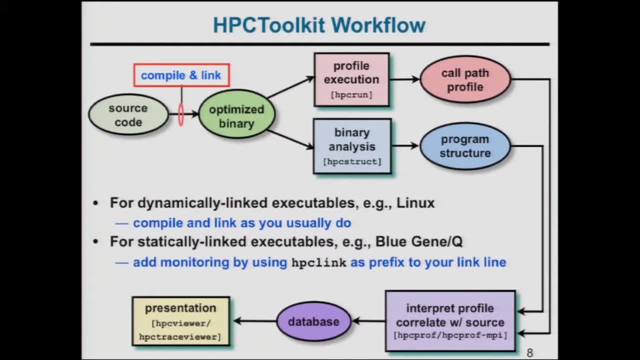 you need to take the code for the performance tool and link it in your application, And for that we have this tool called HBC Link that you add as a prefix to your application. So you just put it in the link line of your make file. 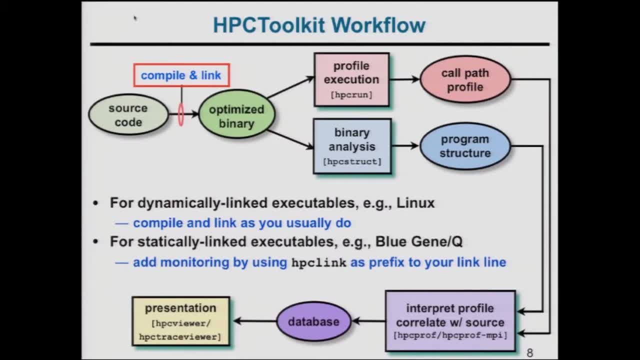 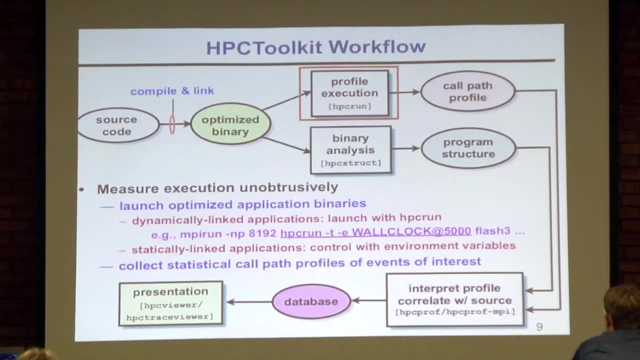 You just say HBC Link and then your normal compile command after it, and that's all you need to do. No compiler wrappers, no serious changing of your build process. Then the second thing you do is, once you've got either your dynamically linked executable- 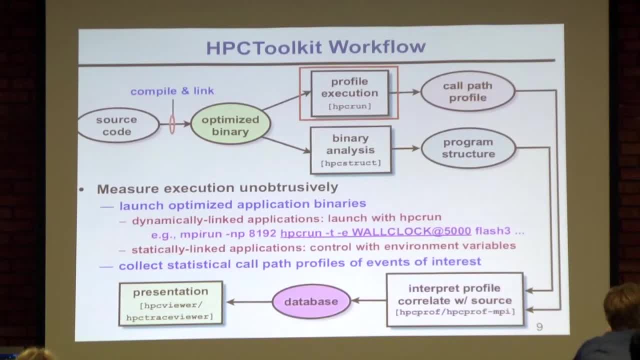 in which case you launch it with our HBC Run tool, And so in the middle, there's an example here that shows how to use HBC Run, How to use HBC Run with MPI, And so you can launch your MPI job. 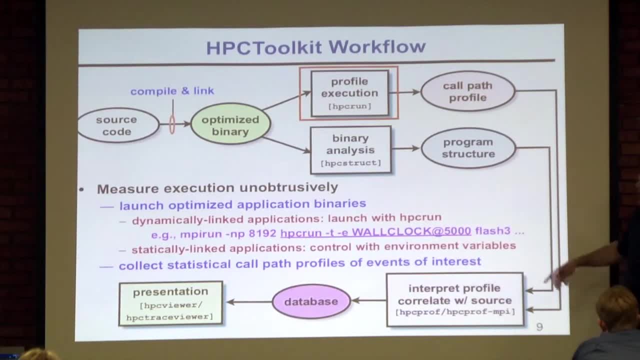 And so here we're launching a copy of Flash 3. And then you just say HBC Run, And then you say what event you want. So this is: I want to measure wall clock at a period of 5,000 microseconds, And then I also want to collect a trace. 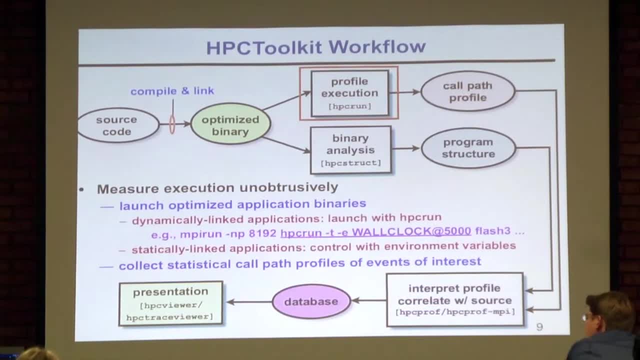 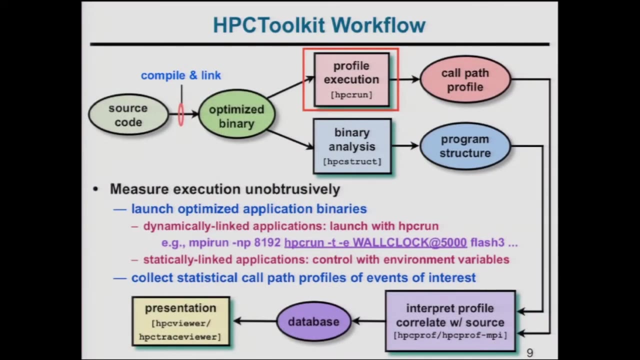 And I just insert that into the middle of my MPI Run command and then it will collect information about every process In the execution. If you're doing this with statically linked applications, then the information about what events you're using, say, the wall clock, and that you're doing tracing. 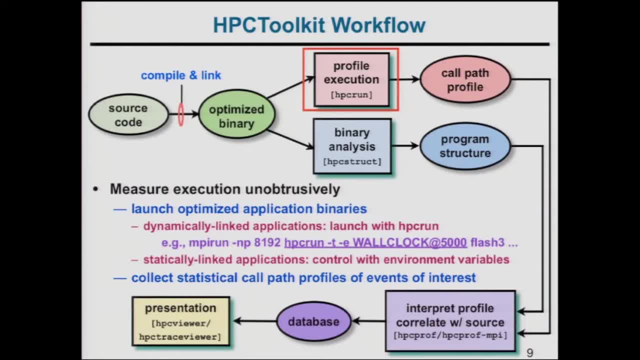 instead you set that in environment variables, because we don't have a way to pass them on the command line, And so when the program executes, then you collect statistical call path profiles of the events of interest, And so I'll say a little bit more about what I mean by that. 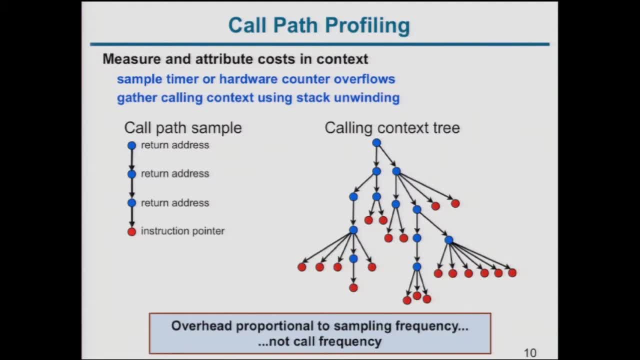 So with call path profiling, what you're doing is you're measuring and attributing costs in context, So you're setting up a timer or a hardware counter to periodically overflow. So what happens is the timer or the hardware counter will go off and it will trigger an interrupt. 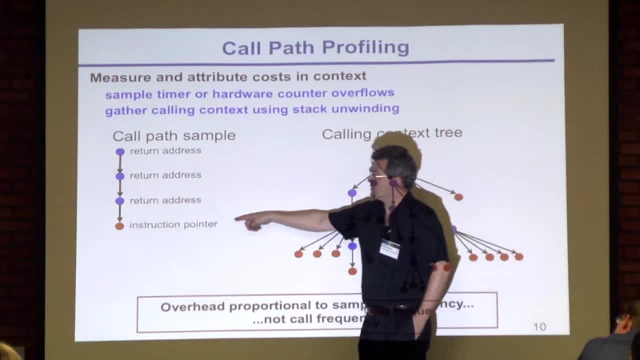 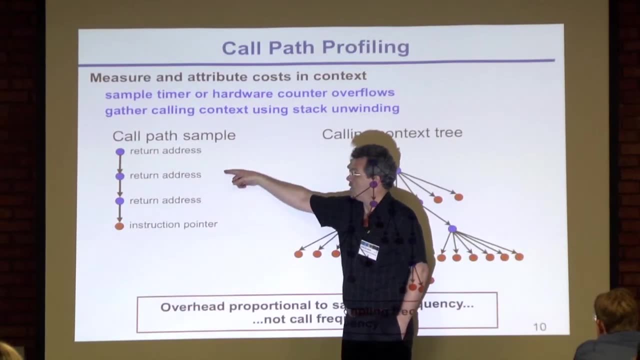 And we'll find out that we're at some program counter location. and then we want to know that I was in some routine C, when called from B, when called from A, when called from main, And so that tells me exactly where the costs were incurred. 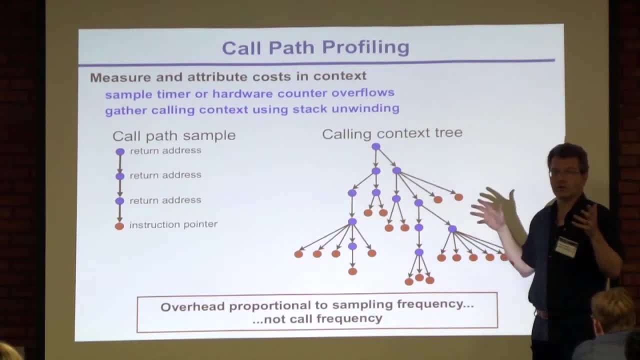 And so if I have an application that's got MPI all over it, knowing that I'm in MPI weight doesn't really do me much good. What I need to know is which MPI weight is a problem, And so the calling context is really important to collect. 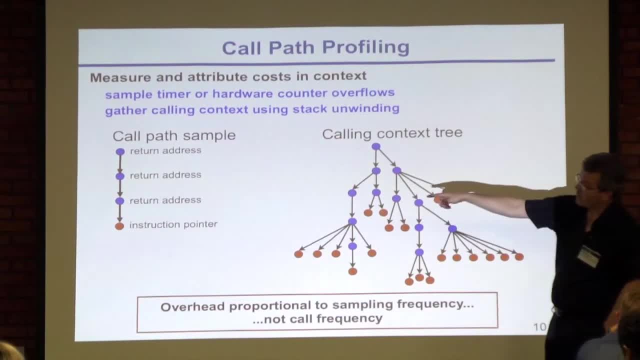 to understand where your problems are, And so that's what happens for an individual sample. when we get an interrupt, We find out where you were, and we attribute the cost to the context, And then, over the entire execution, we'll collect up something that we call a calling context tree. 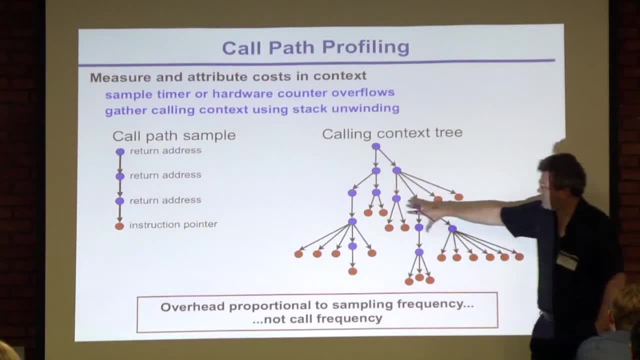 And so conceptually you can think of main being up at the top, and then this might be the initialization phase and this might be the solver phase, And all the interior nodes represent routines or call sites, and then all of the leads here represent where costs are incurred. 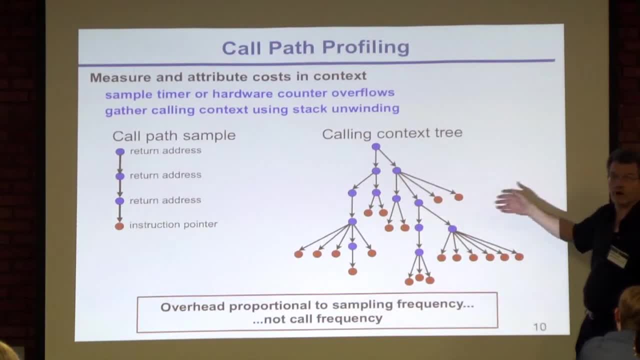 And so what we're collecting is a tree with weights on it during the execution, And the important thing is that collecting this information is proportional to the sampling frequency, not the calling frequency. So it doesn't matter whether you have small procedures, It just matters what you set as your timer period. 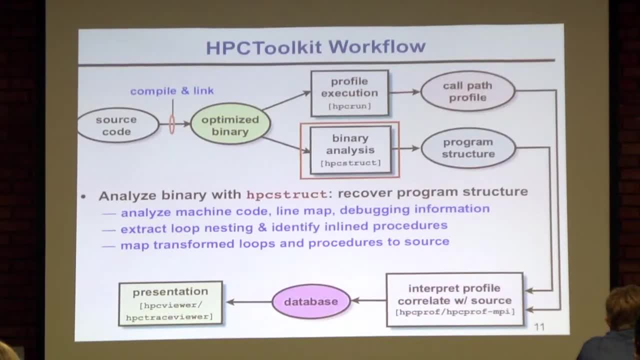 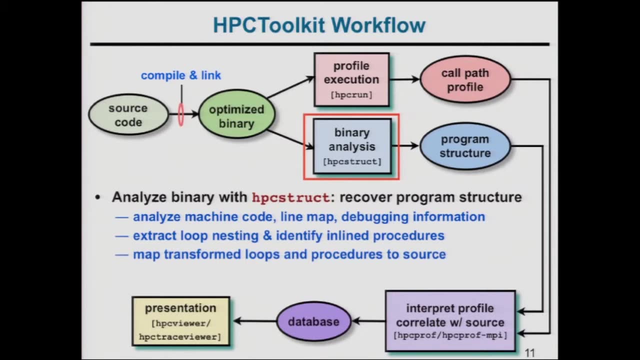 or your hardware counter period. So then the next thing you do is you run our HPC struct tool And what this does- this is a unique tool to HPC Toolkit, So it does binary analysis of your executable, And so we analyze it. 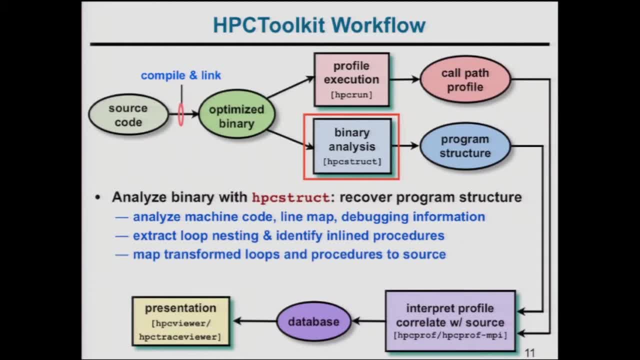 So we analyze the machine code, We parse the machine instructions, We rebuild the control flow graph for your code, We figure out where the loop nests are, We identify inline code, We figure out what statements are inside loops, And so this isn't the source code view. 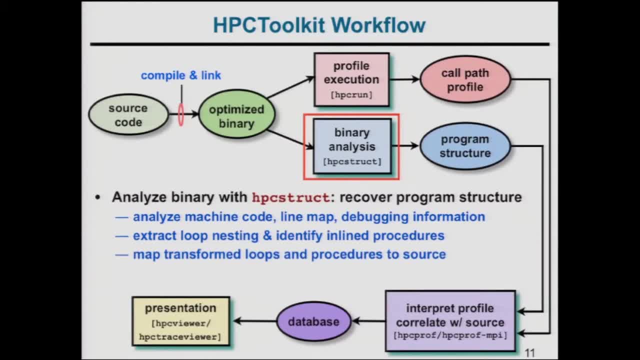 This is actually how the code is going to execute. So you might have several Fortran 90 statements that are adjacent in the code, and if the compiler fuses them all into a single loop, you'll see that That's what comes out of our binary analyzer. 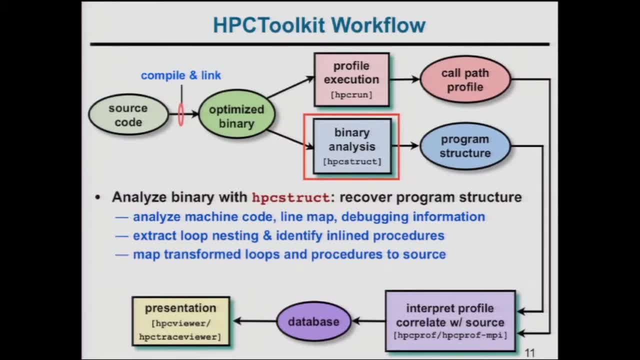 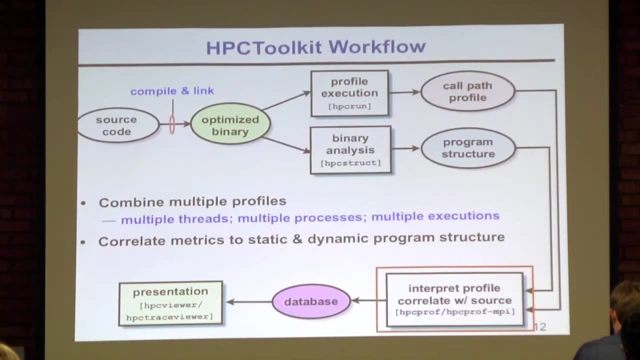 It will tell you about these fused loop nests, And then it maps the transformed loops and procedures back to the source code, And so we use this information, along with the call path profile, in order to interpret the measurements that we've made. So then, once we have our call path profile, our dynamic measurement, 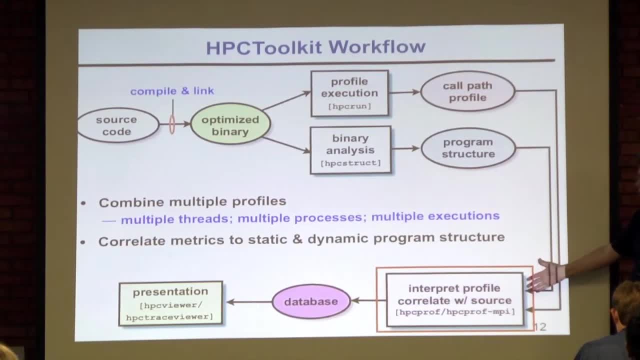 and then we have our static program structure. we have two tools that combine them. So there's HPC Prof, There's HPC Prof and HPC Prof MPI. And so what HPC Prof does is it runs on the head node and it will combine multiple profiles or multiple trace files. 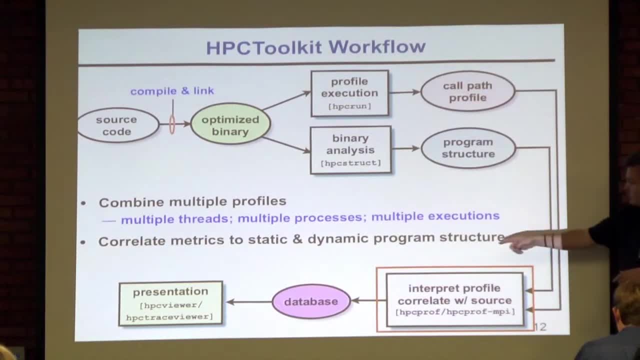 and knit the results together into this performance database. And then HPC. Prof. MPI is for dealing with large-scale executions, where you launch this as a batch job and it's going to analyze your performance data in batch, And so that's when you've got thousands of profiles. 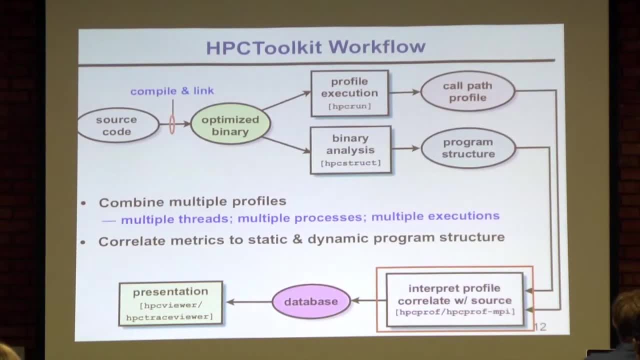 and you don't want to wait a couple of hours while it analyzes on the head node. You can just launch a job and analyze it in minutes. So what this enables you to do is to combine information about multiple threads, multiple processes, multiple executions. 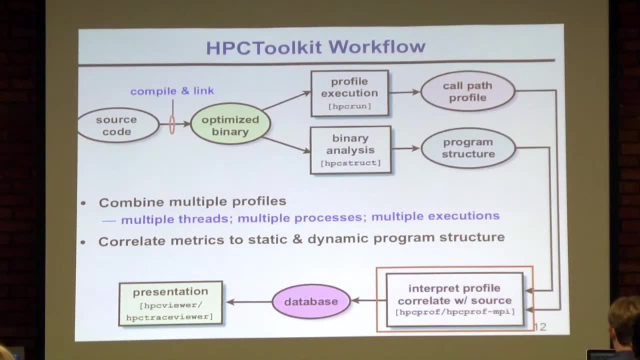 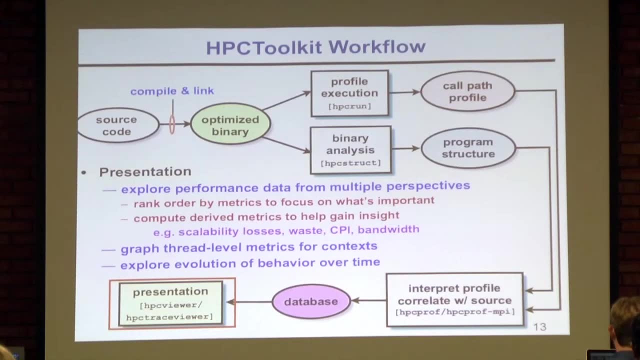 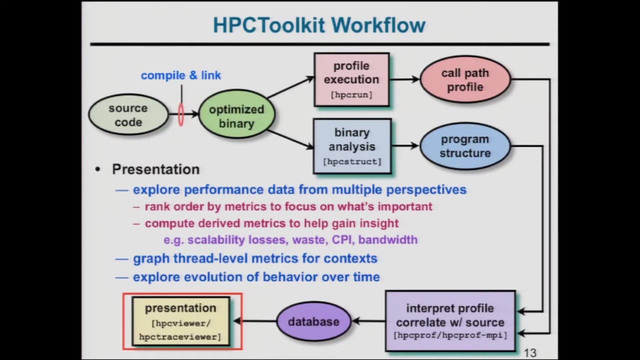 and then correlate everything to both the static and dynamic structure. So then, finally, we have two presentation tools. You can explore the performance data from multiple perspectives. You can rank all the metrics by what's important, So you can say: I want to see the procedures where I spend the most time. 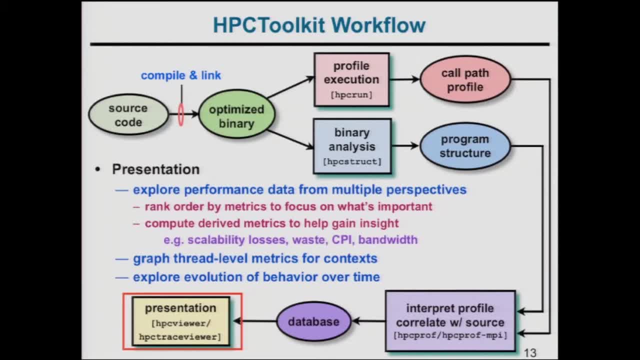 sort it up at the top, And so this is to try and deal with information overload. If you've got really big applications, what you really want to do is just focus on what's important And so, sorting you get to define your own metrics. 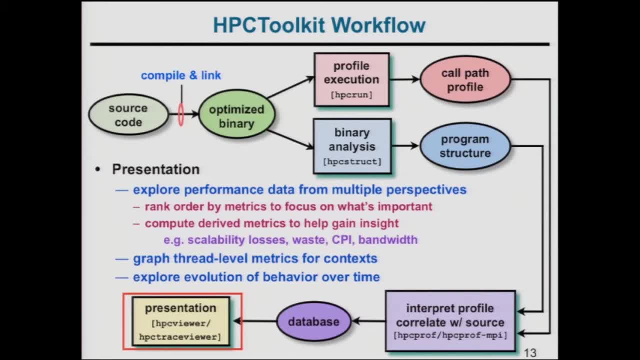 and you get to sort by them, and that lets you focus on what's important. So we can see something from a code-centric view, from a thread-centric view And also from a time-centric view, and I'll show you what these tools look like. 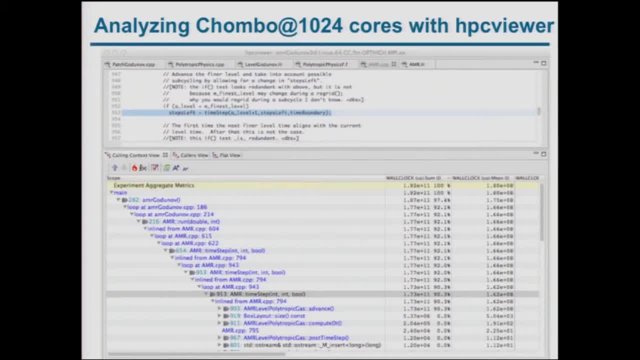 So I understand from my student, Kartik, that you had a little bit of exposure to Chombo over the last week, And so what this is showing is the HPC viewer view of a 1024 core run of Chombo, And so what we have here, it's a little bit washed out on the screen. 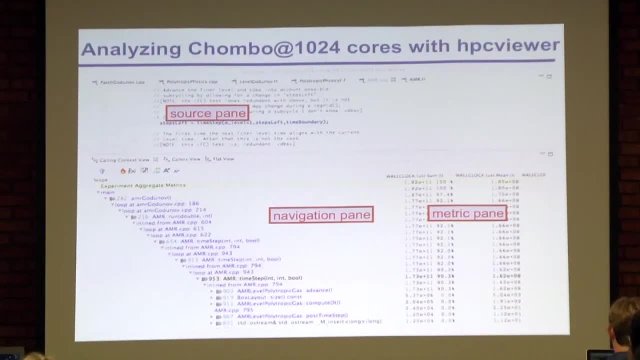 There's three panes: There's a source pane, up at the top, There's a navigation pane, And so what this is showing you is elaborated call chains, And so what we did is we took these calling context tree for all of the 1024 cores and we mashed them all together. 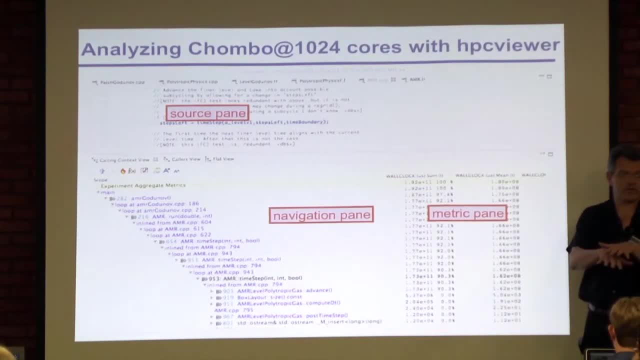 And now we're looking at where you spent your time across all of the 1024 cores sort of summed together, And we have summed metrics and mean and min and max and whatnot, And so you can look at these, You can look at these statistics across all of them. 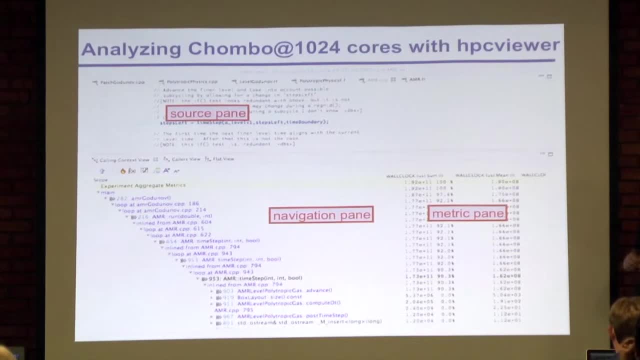 And then you can also graph data across the individual cores as well, and I'll show you that in just a minute. And then so we have our navigation pane, And so if I select something over here, then I'll find the source code will come up that corresponds to it. 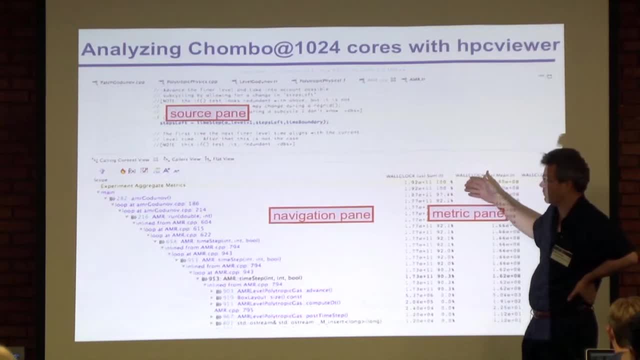 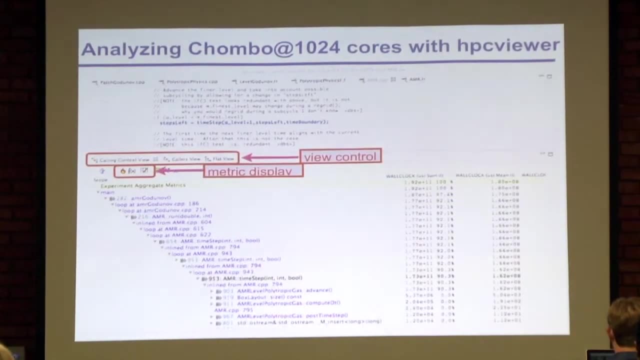 and I can sort by these metrics to see what's important, And there's several different views here. There's some view controls So you can look down call chains, You can look up call chains or you can look at flat, And I'll say a little bit more about that on the next slide. 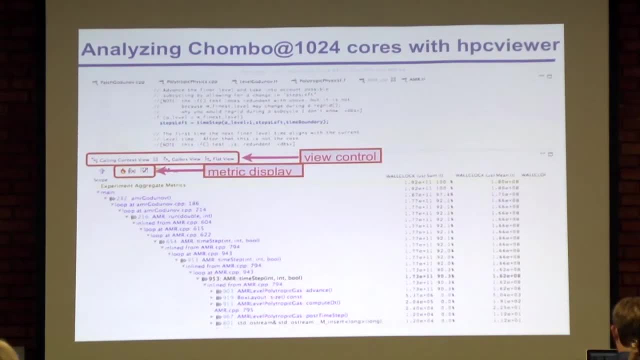 And then there's also some control for computing derived metrics, or if you've got lots of metrics columns, you can just hide them so that you can just focus on the one or two that you care about. You may have one that's sort of scrolled way off the screen. 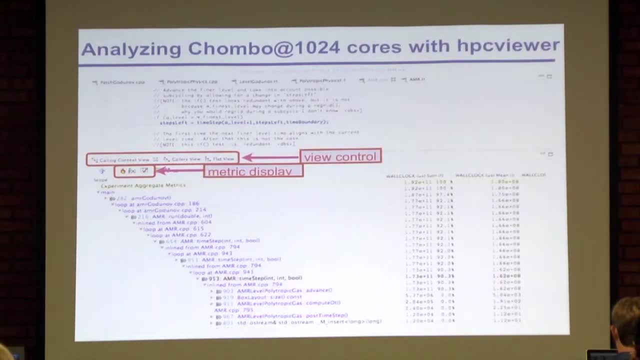 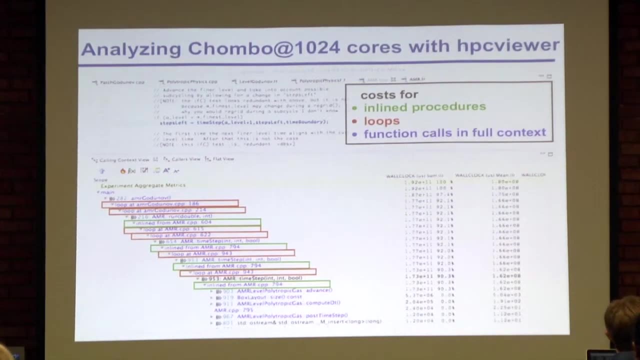 and you can move it over to the left where you can see it, or hide everything else in between. And then the thing that you get with HPCToolkit, which is a consequence of using this HPC struct, binary analysis, is not only do we get call chains, 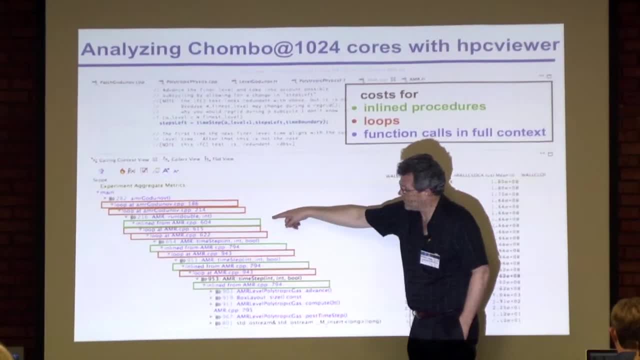 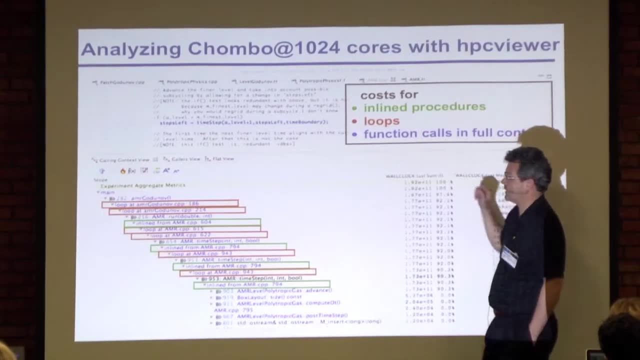 but we also get information about loops in call chains, And then the green here shows that there's inline code as well, And so not only do we see the call chains, but we see the loops and the inline code that's in the call chains. 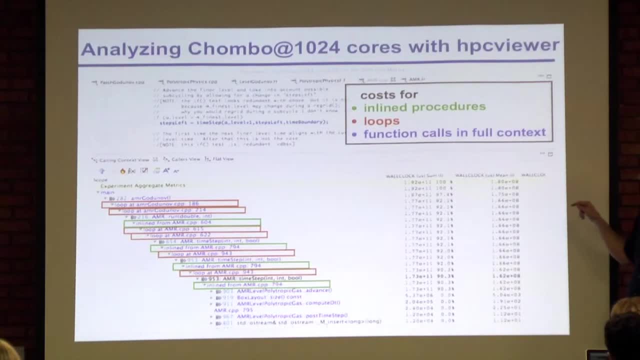 and we get that from our binary analysis, where we're recovering loops and information about inline code, And so this costs nothing because essentially we're collecting these dynamic call chains at runtime and then we're just overlaying this additional information we got from static analysis. 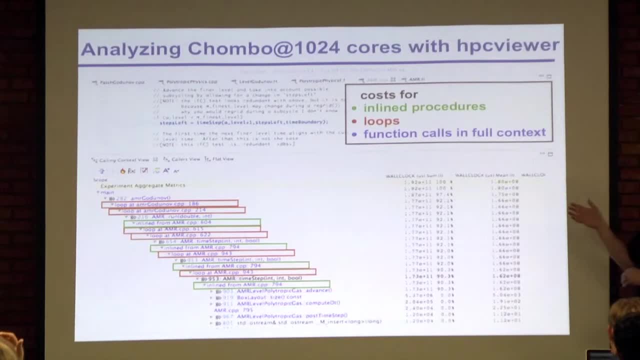 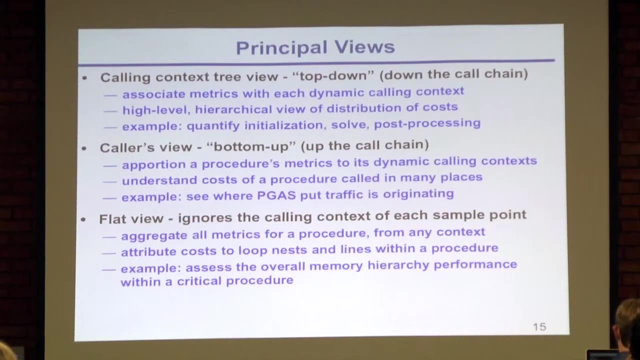 So it doesn't cost anything to collect at runtime to give you loop-level performance information. So I mentioned that there are three different views. So the calling context view: you're looking down call chains and so that's good at seeing things like how much time that I spent. 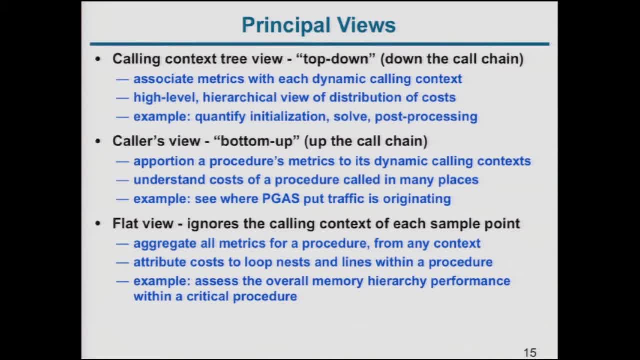 in the initialization phase or the solve phase or the post-process phase. The caller's view, where you're looking up the call chain, is so. I spent 30% of my time in MPI weight and there's lots of different MPI weights in the program. 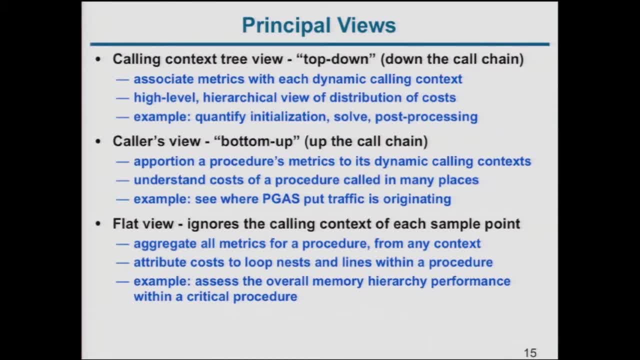 and rather than searching down the call chain and trying to find them all, you say looking up from MPI weight, I spent 30% of my time here, so let's look at the different places it's called and which ones are most important. 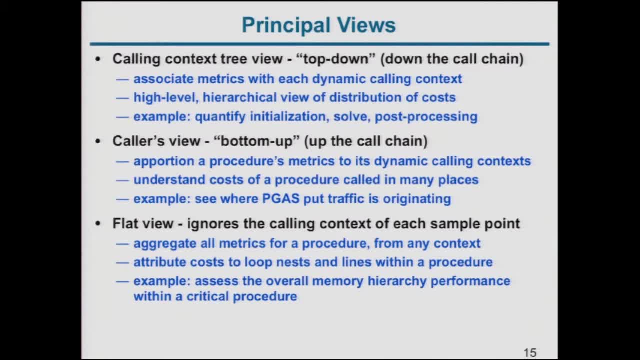 So that's looking up the call chains, And then the flat view says: well, so I don't care how this thing was called. What I want to know is how much time was spent in here. and let me look at the loop nests in this procedure. 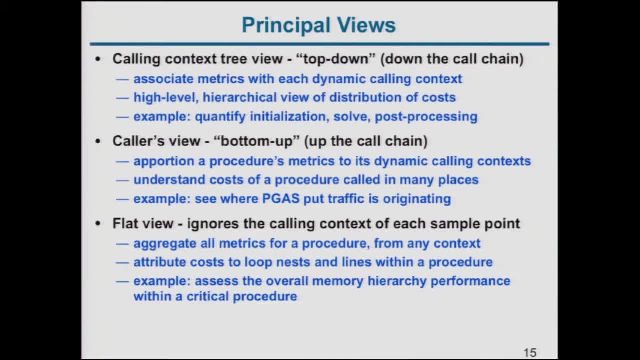 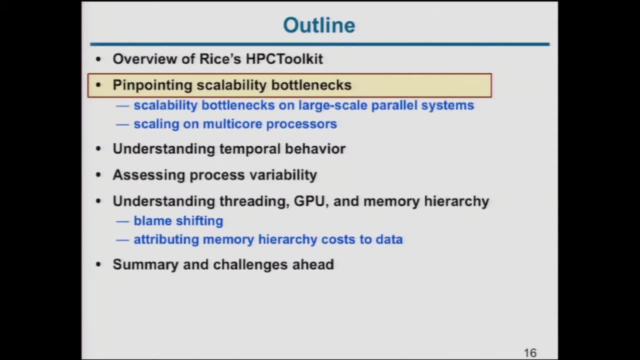 And so you can see just sort of what's important in the procedure when it's used, from all of the contexts in the program. Okay, so then how do we use these tools? So let me talk about pinpointing scalability bottlenecks, since that's something that's relevant here. 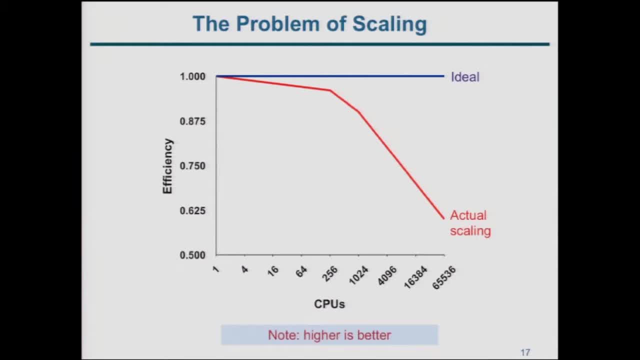 So the problem is that as you scale to larger numbers of processors, now this is a problem. This slide was made several years ago, and so this is only scaling out to 65K, which I guess is sort of a toy system these days. 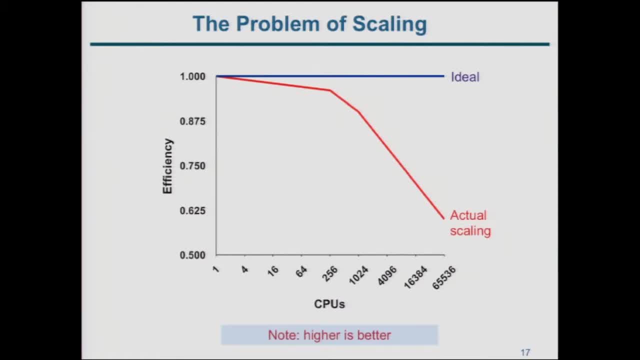 So what you want is, as you add additional processors, what you want is your parallel efficiency to be one. So as I double the number of processors, I want, double the performance, And so, if I'm running it on a fixed-size problem, I want my execution time to half. 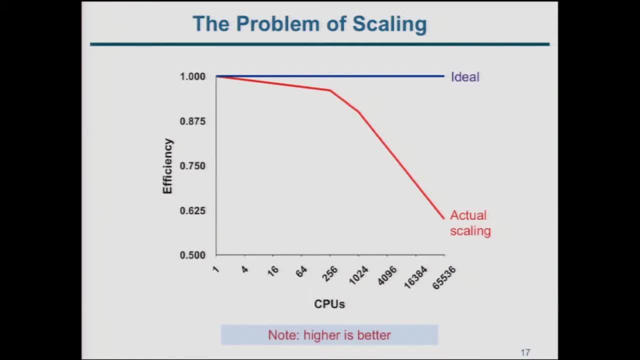 And so, actually, when you run on a larger system, what you'll find is often- it's often the case- that your actual scaling tapers off, and so you're not getting the full benefit of every core, And so what you want to know is: what's the gap? 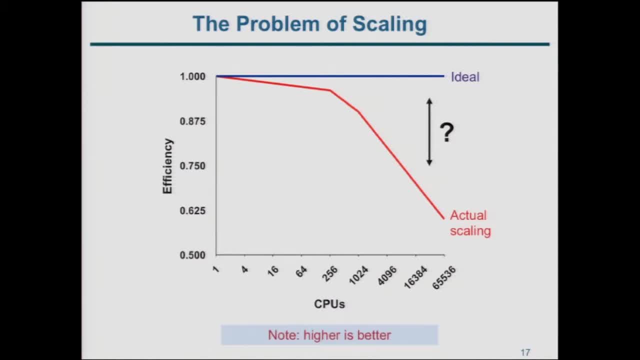 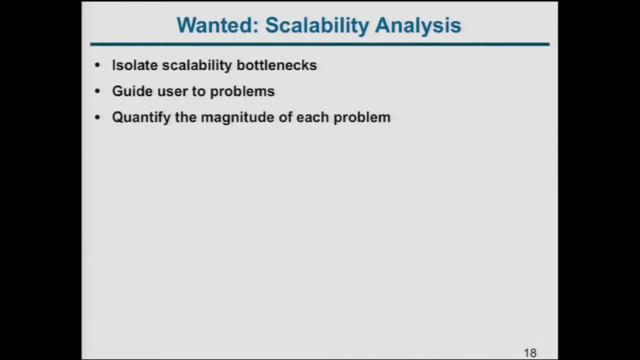 and where is it in my program and how can I fix it. So you want to be able to isolate scalability bottlenecks, figure out where they are in your code and then quantify the magnitude of each problem, And so that's something that we've solved here. 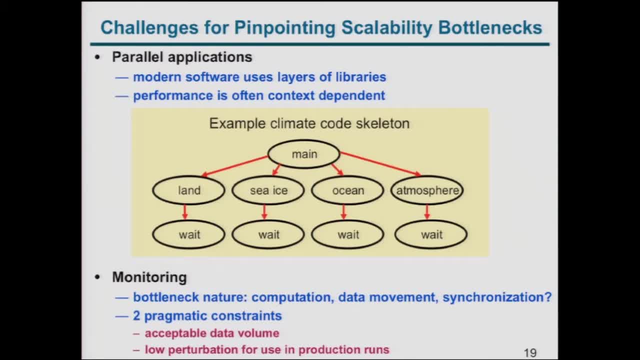 So the challenge for pinpointing scalability bottlenecks is: you've got lots of different layers of software. So let's say we have this climate code here. So there's a main program and it's calling a land simulation, a CI simulation, ocean simulation and atmosphere simulation. 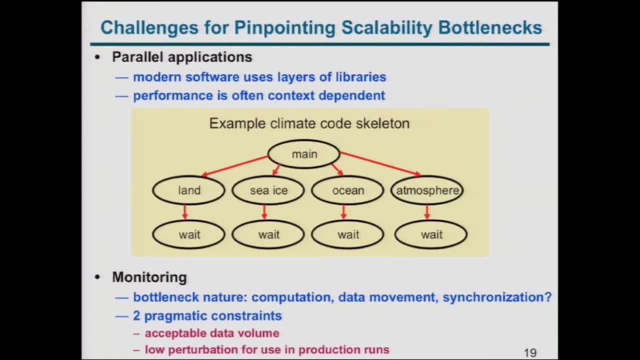 And then this calls to MPI weight down in each of them, And so we need to be able to know which of the MPI weights in the program is a problem. So we need to understand the context And then, when we're monitoring, a challenge is: 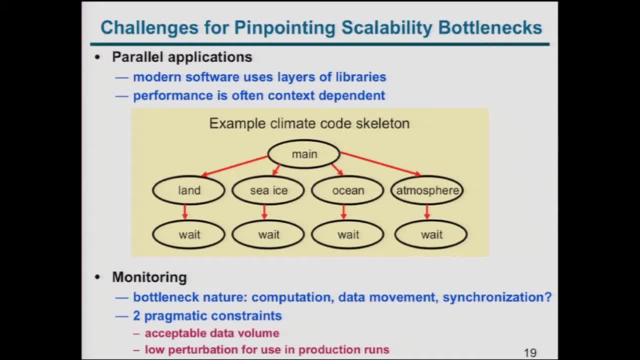 well. we want to be able to identify bottlenecks, whether they're due to computation, data movement synchronization or whatever Replicated computation, And the pragmatic constraints are that we can't collect a huge amount of data and we don't want to perturb the execution. 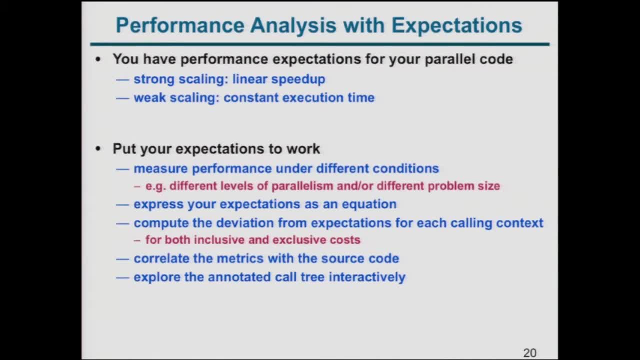 So how are we going to do this? Well, the idea is really simple in hindsight, So you have some expectations about what's going to happen with your code. So I suppose you talked about strong scaling and weak scaling previously. Is that true? 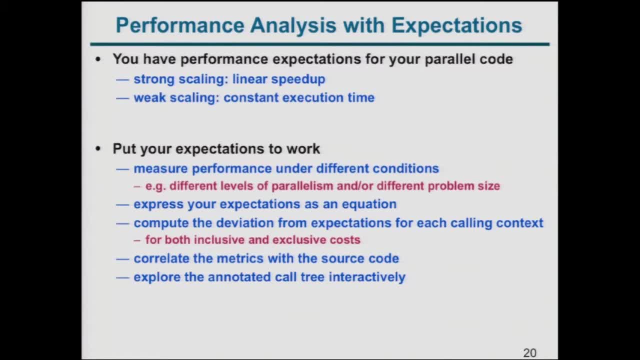 Okay, I'll review it briefly here. So with strong scaling, when you're taking the same size problem and then you run your application on a larger number of processors. With weak scaling, when you double the number of processors, you double the size of the problem so that each processor 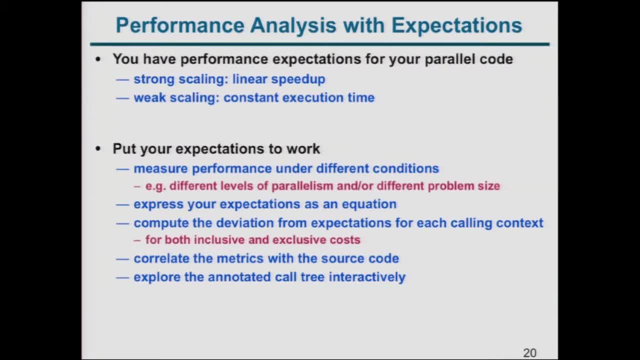 has a constant amount of work, And so those are two different ways that you might scale your code So you could take your fixed size problem and then keep running it on larger and larger numbers of processors and say how come I'm not getting the full benefit. 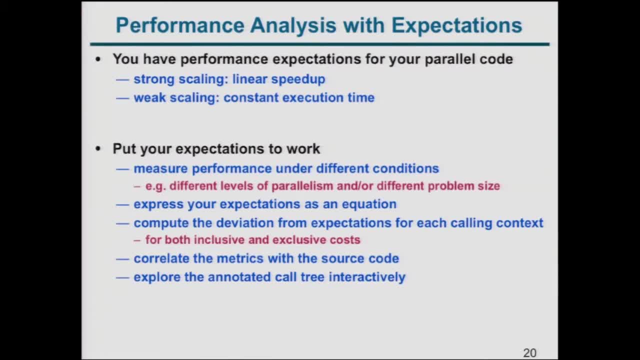 Or you can take your weak scaling problem and you say, well, I run it on a problem of size K on so many cores. Now I double the number of cores and I double the problem size and I want it to run at about the same time to get a higher fidelity simulation. 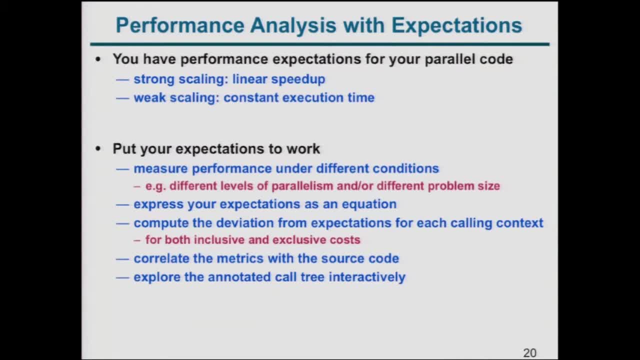 And so in either of those cases, you have some expectations of how the performance is going to work out. So, if you're using strong scaling, when you double the number of processors, you expect it to take half the time. When you're using weak scaling, you expect it to take the same amount of time. 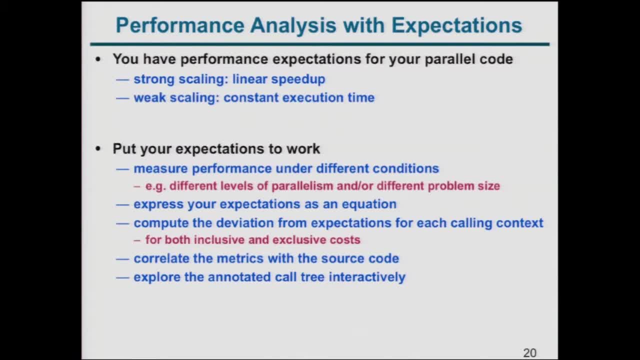 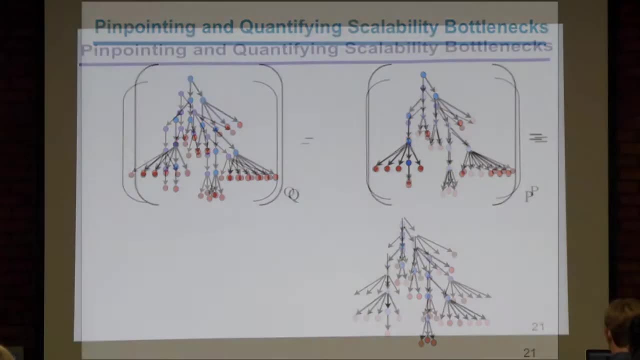 And so you can express your expectations as an equation and then compute the deviation from your expectations in every calling context in the program, And then our tool can correlate all that with the source code and then you can explore this interactively. So here's the idea. 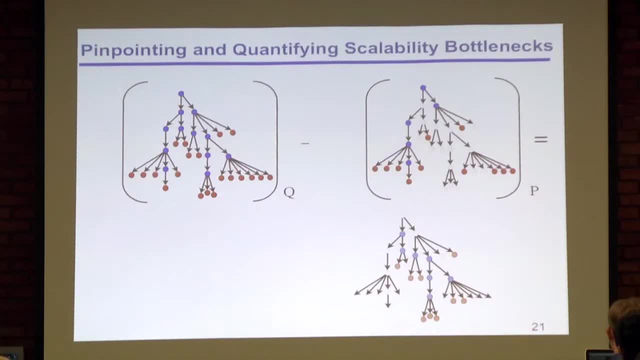 So let's say we collect this calling context tree on P processors And so I've shaded the nodes a little bit to indicate sort of the weight that was associated with each of the nodes, And so we have some weights on the tree saying this is our cost. 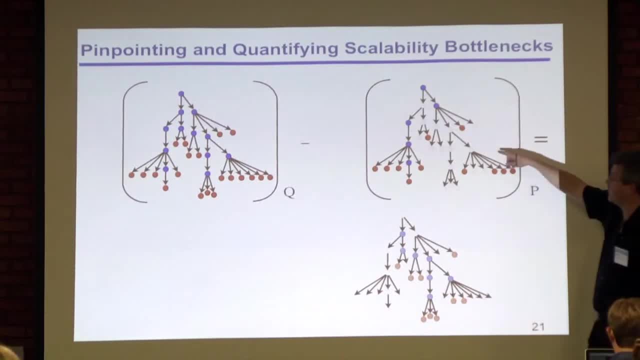 at each of these places in the calling context tree And then we collect it on a larger number of processors and we get a different set of weights, And so then we can difference the two and say what's the difference between them. So it might be that in the small scale execution I spend 400K units of time. 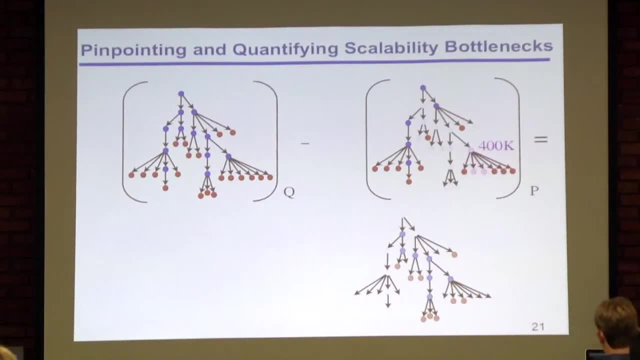 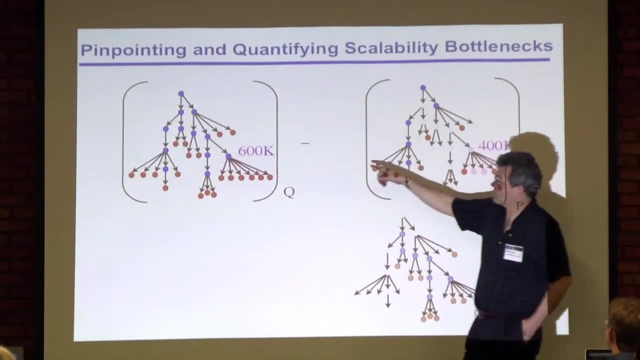 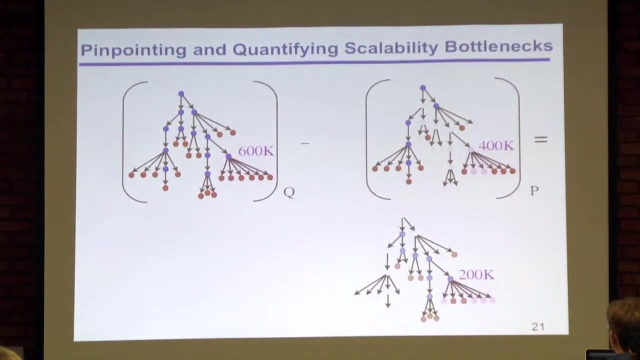 in the solver You can't really see the pink highlighting with this projector, And then in the larger scale execution, you may spend 600K units of time in the solver over here And then. so what that gives you is the difference of 200K units of time. 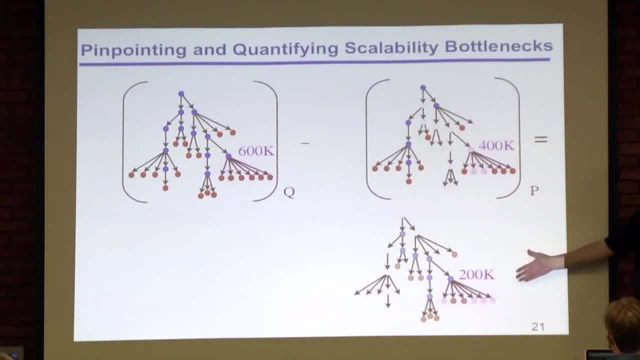 And so what this amounts to is wasted effort. And so if we take this wasted effort and we divide it by the total effort that we put in in the entire execution, we get a fraction of wasted effort. That's telling us why we're deviating from that perfect scaling. 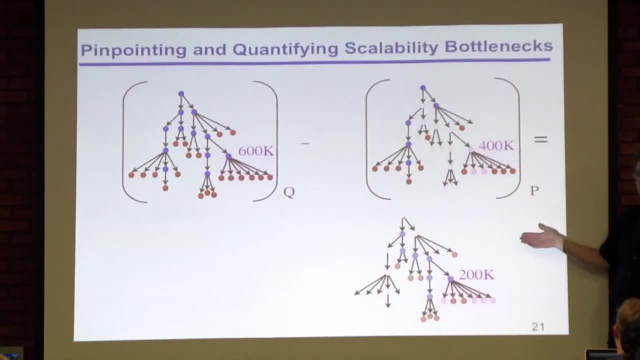 And with our fraction of wasted effort. that's also the same thing as scalability loss. So we take our fraction, we multiply it by 100, and now we're looking at our percent scaling loss. So this works for strong scaling as well. 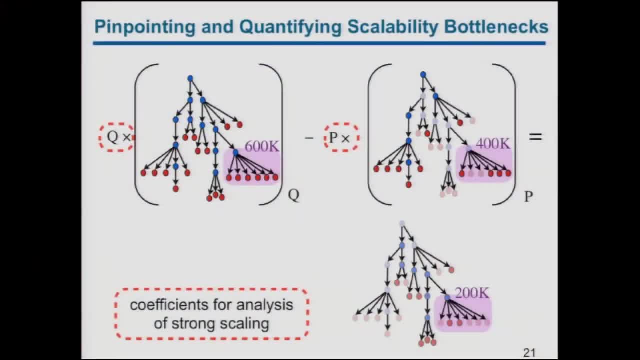 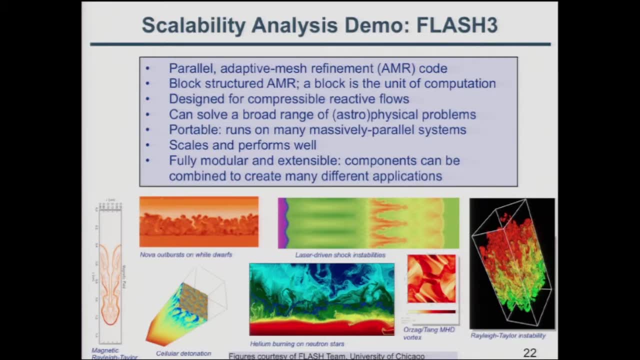 You just have to throw a couple of coefficients in front of the equation. So let me show you how this actually works. So this is for the flash code that was talked about before lunch. So it's a structured AMR code And this is a simulation of a white dwarf detonation. 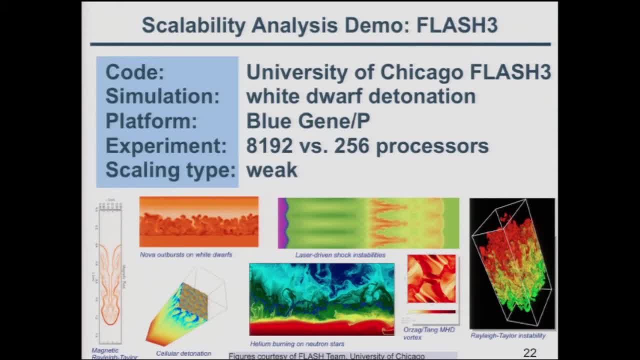 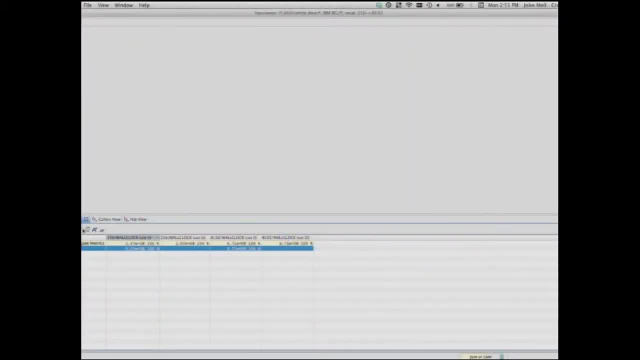 And we're comparing scaling of 256 cores to 8K cores on a blue gene P system. Okay, This is going to be a little bit small, but I think you'll get the idea anyway. So what we have here is there's a calling context tree in the navigation pane. 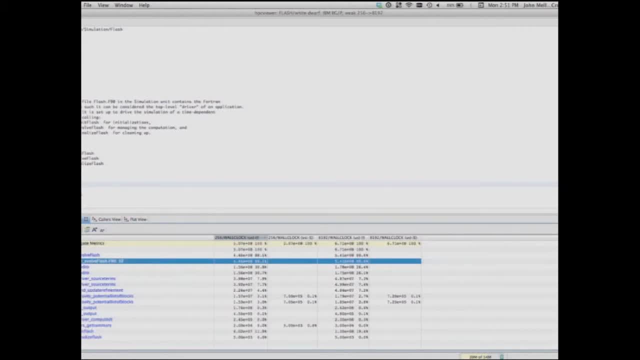 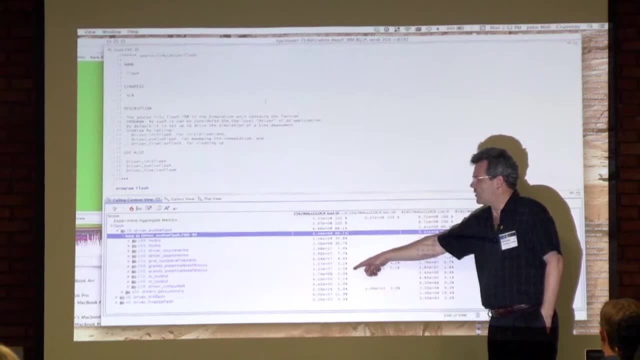 And so right now I'm looking at the root of the calling context tree. So what we have here are a couple of columns. We have results, measurements of where we spent our time on 256 cores, where we spent our time on 8 cores. 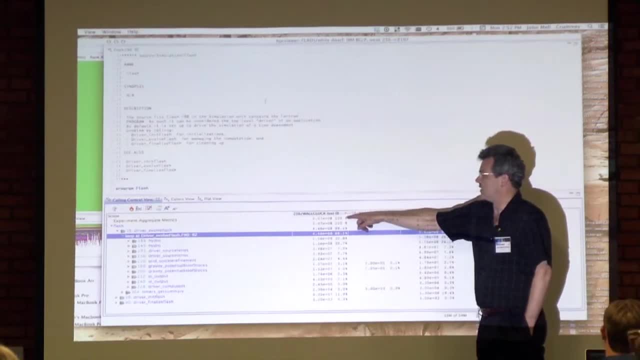 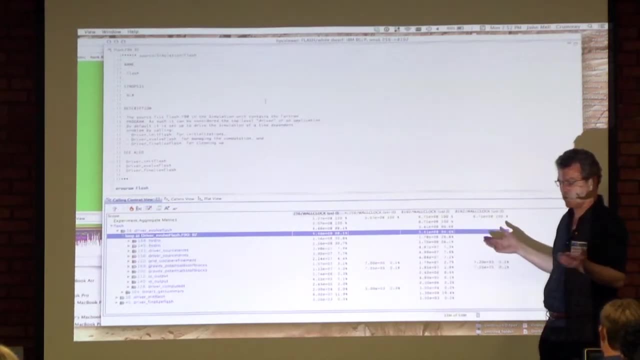 This is a weak scaling experiment, And so we expected the time to be exactly the same on 256 cores as on 8K cores, because as we increase the number of cores, we proportionally increase the size of the problem, And so this is larger than that. 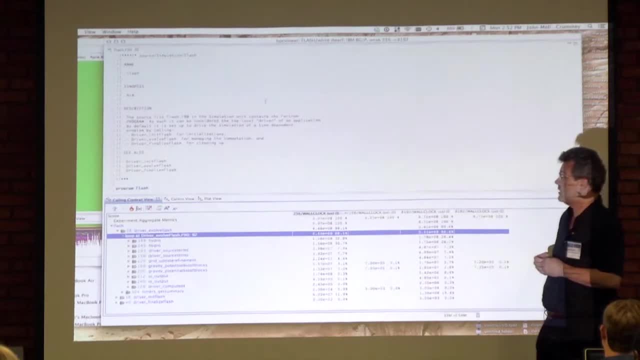 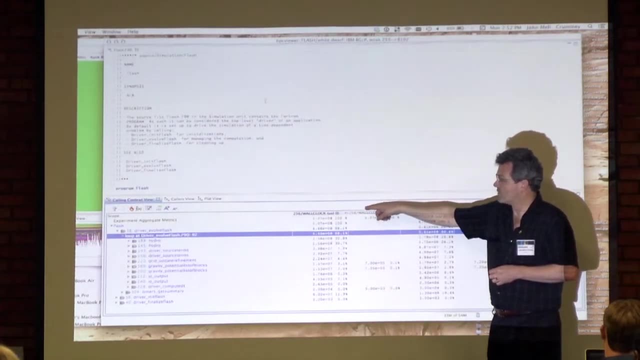 which means that we have some scaling loss and we want to find out where it is, And so, with our tool, we can dig through and we can look at where we spent our time for 256 cores or where we spent our time for 8K cores. 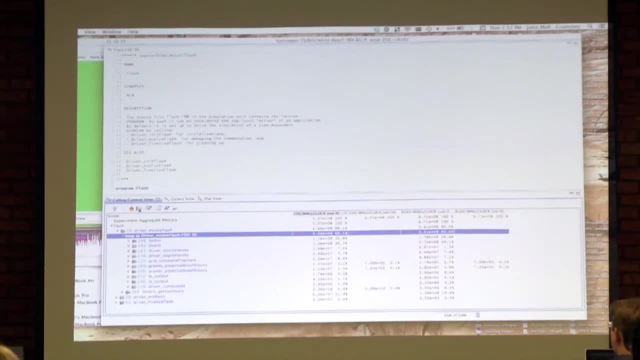 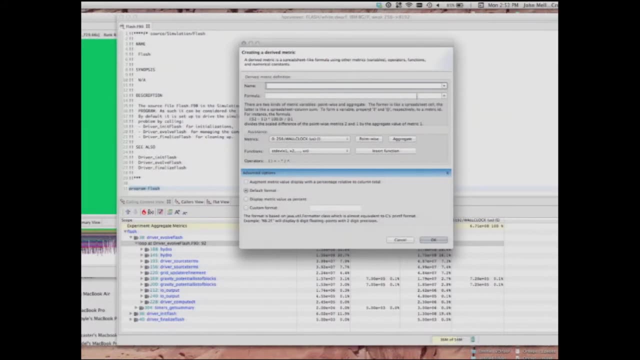 But the real power comes from comparing these two different executions. So I have a spreadsheet, like I pressed a little function button and that lets me define these little spreadsheet-like equations, And so I'm just going to pull the equation out of the hat. 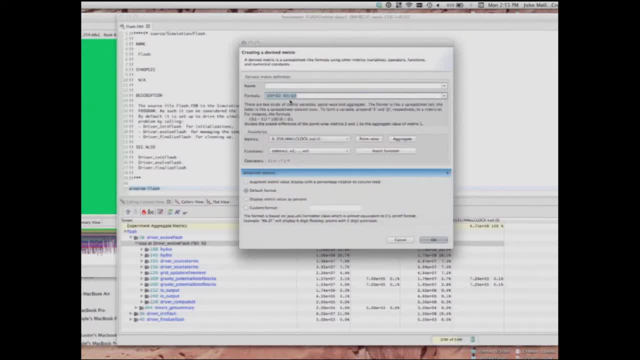 And so it's actually doing the same thing that I showed you earlier. It's differencing the cost in the two trees, It's dividing by the cost that's associated with the inclusive cost associated with the root in one tree, multiplying by 100.. 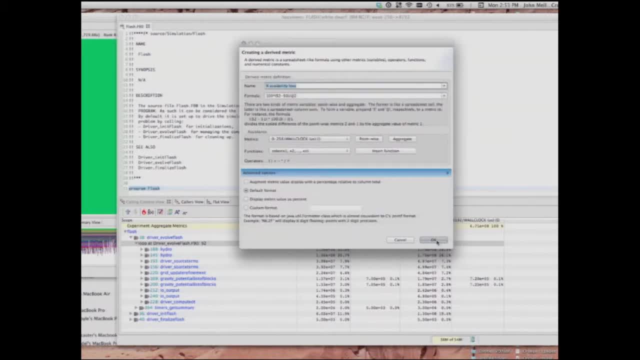 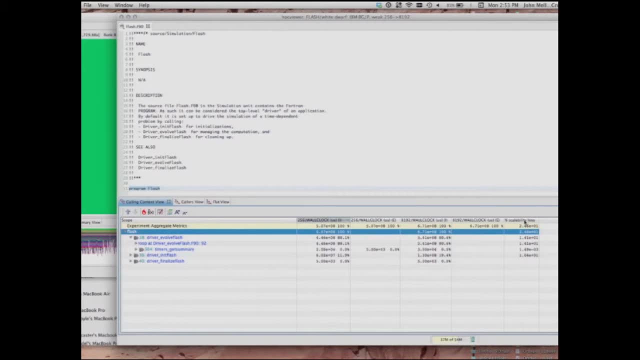 And then that gives me percent scalability loss, And so I was careless in the work The way I clicked this, and so it gave me the number in scientific notation. I can make it come up without scientific notation, Okay, so what this says is that I have a 24% scaling loss in my execution. 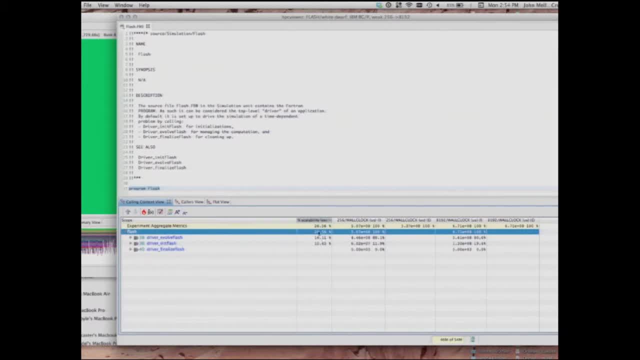 And if I look I can see that of that 24% scaling loss, that most of it is in the evolve flash phase and 14% in the evolve flash phase and 10% in the init flash phase. And so I can say: 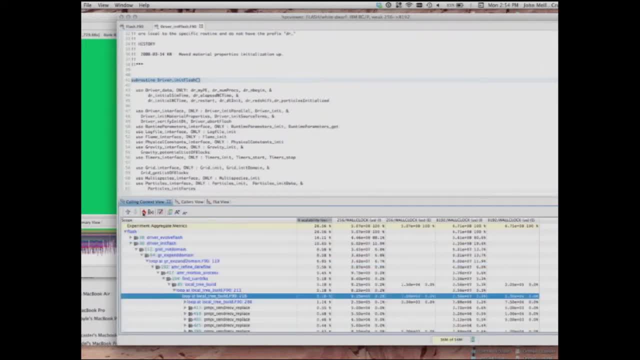 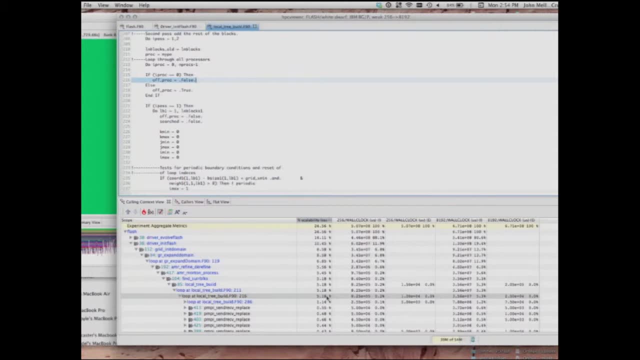 well, show me where the scaling loss comes from, And it will drill down through the call chains and it finds a loop nest And it says that this loop nest is associated with 5% of a 5% scaling loss, which is one-fifth of the scaling loss for the entire program. 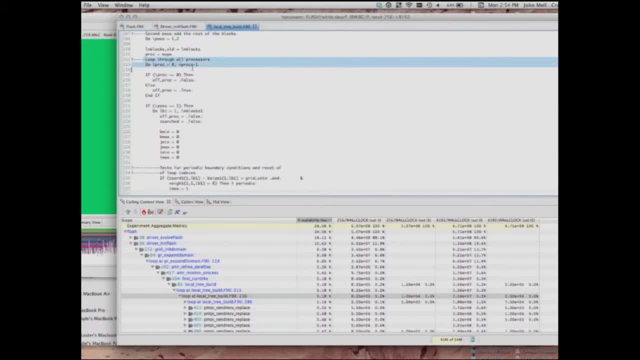 And right above this, it's inside a loop and we see something that says loop over all processors, And so as we increase the number of processors, then this loop is going to take more time. So what it's actually doing here is there's as part of the adaptive mesh refinement. 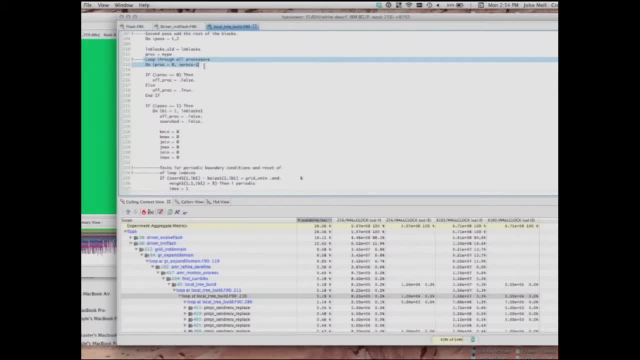 you end up with a block of data, and then there's you need to know which processors have the neighboring blocks of data after adaptive mesh refinement. And so initially what they were doing was everybody said, okay, here's the blocks I have. 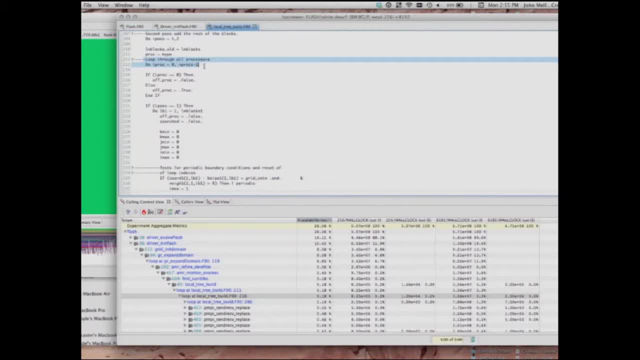 and they pass that information to their right neighbor And then the information circles all the way around the ring. So effectively it's an all-to-all communication. Since it's going around a ring, it's taking p time steps to go around the ring. 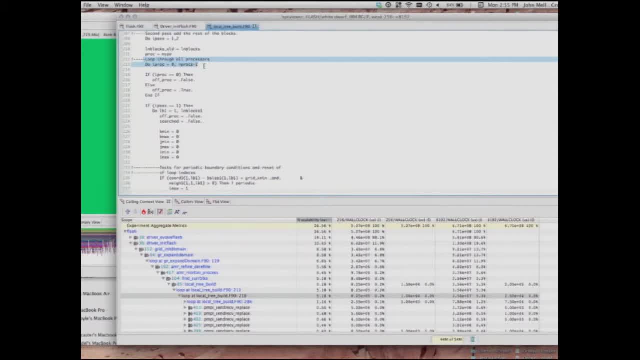 And so as you increase the size of the number of processors, then there's an increasing number of hops around the ring, and so it doesn't scale so well. So that's the one problem here. Now this isn't the only problem. 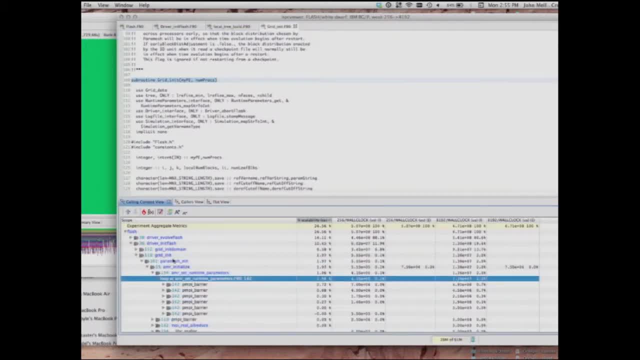 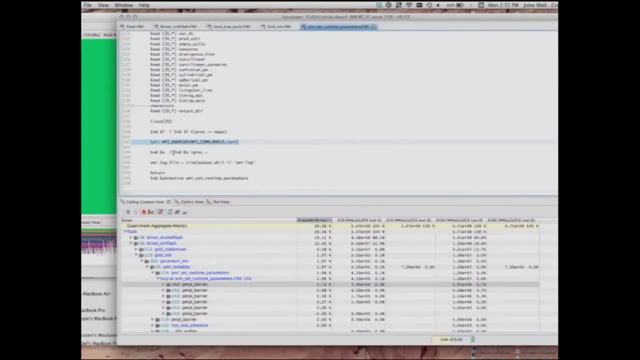 You can look at every individual iota of cost in the application and see where its scaling bottlenecks are. So here's another one where there's an MPI barrier And there's also a suggestive. I'm at the end of a loop here. 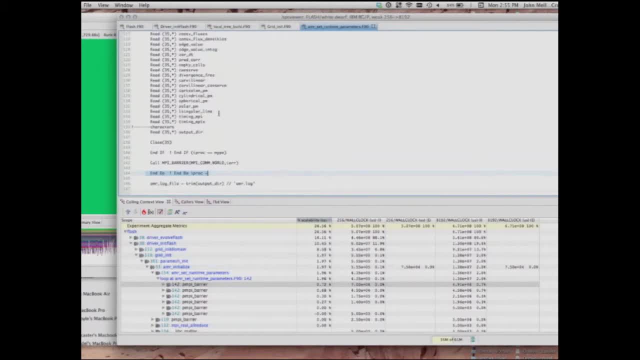 And looking up just a little bit earlier, you see there's IO and it's doing reads and then there's a loop up at the top that says let's iterate over all the number of processors. If it's my turn, I'll open the input file. 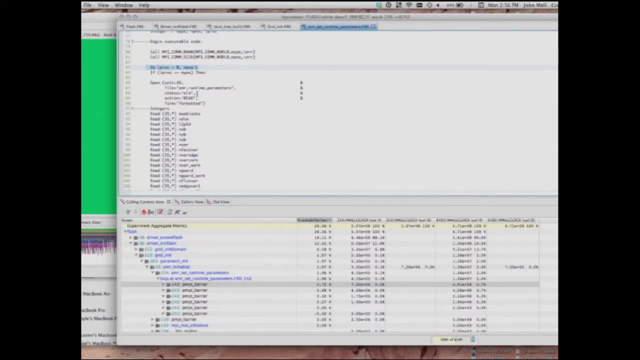 Well, so what happened, I think, was somebody crashed the file system by having 20,000 processors open the file at the same time. It would have been better to just read it and broadcast it. Okay, so that gives you the idea. 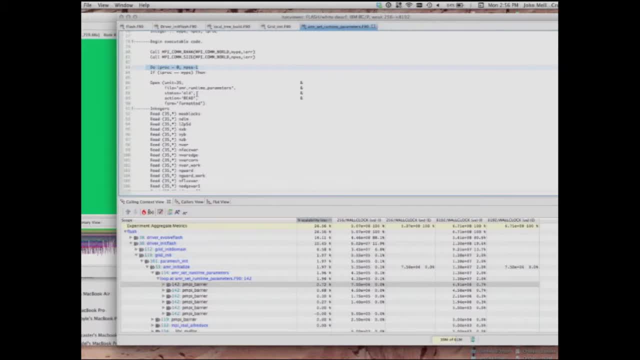 How this tool works. So I'm looking at data from several different executions and doing comparative analysis and it will show me where these bottlenecks are And I can show in the evolve phase that in fact it has the same adaptive mesh refinement bottleneck. 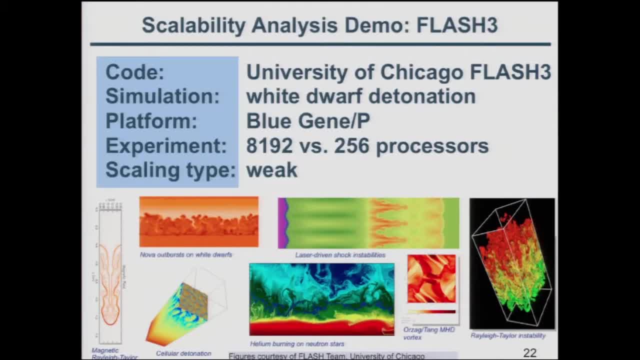 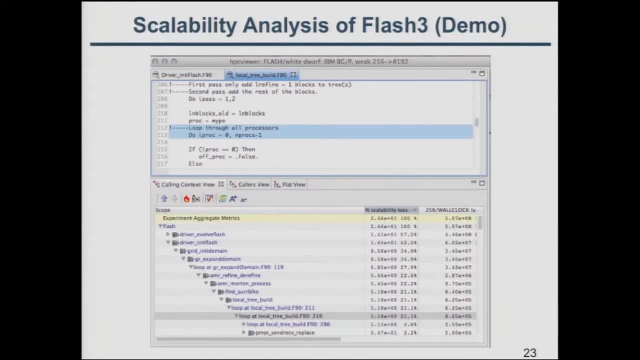 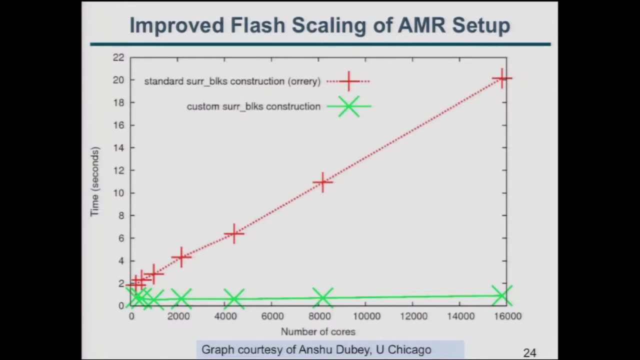 that the other one had in the initialization phase. Okay, so that was scalability analysis across processors, but we can also do it within nodes, So you can run it on. so this is for that case and so this shows that the Flash team. 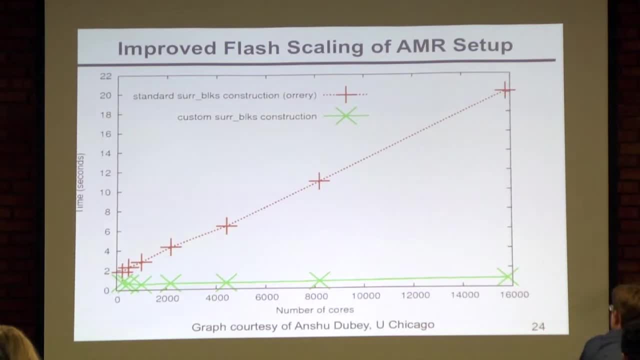 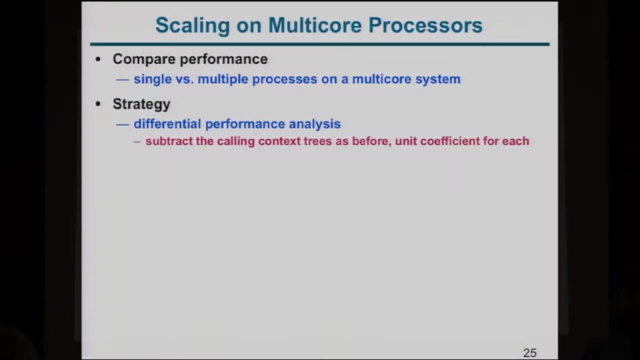 given this information, their execution time used to go up like this for the block construction and then when they fixed their block construction, the scale it was flat and so the flat is scaling. So this is a little while back, So you can also do the scaling on multicore processors. 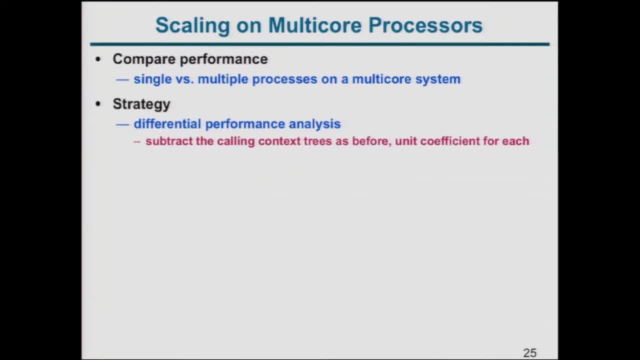 So if you're running on, say, four cores and then you scale up to run on 16 cores, you may find that there's not enough bandwidth to main memory, and so that may be a bottleneck. So you can compare a four-core run versus a 16-core run. 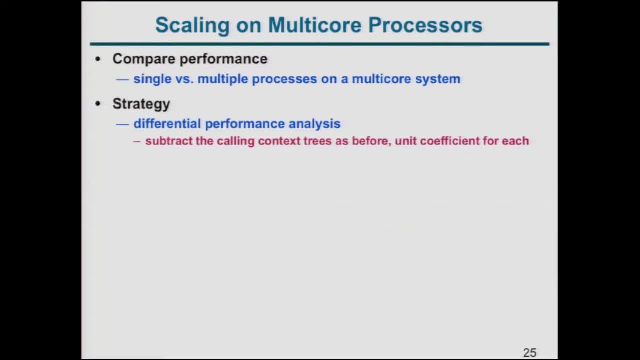 or you can use simultaneous multithreading and use more hardware threads than cores. So use two threads per core or four threads per core and look at the scaling within a node. And so you do the same thing. You just subtract the calling context trees, just like I did. 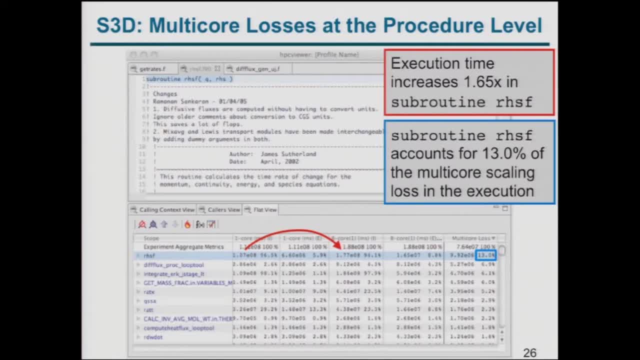 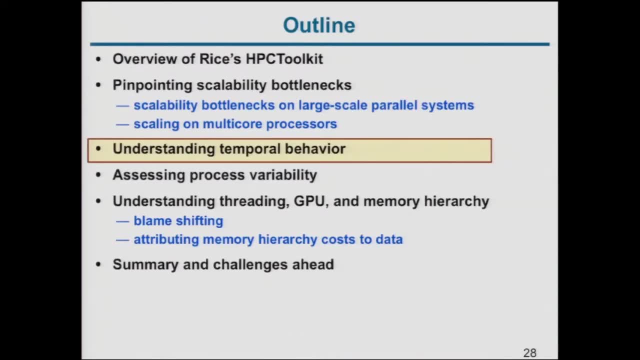 and it can point out the routines in the code where there's the worst scaling, or even individual loop nests where there's the lowest scaling. So another thing that we do is we use sampling to understand the behavior over time, And so this is very different than the tracing. 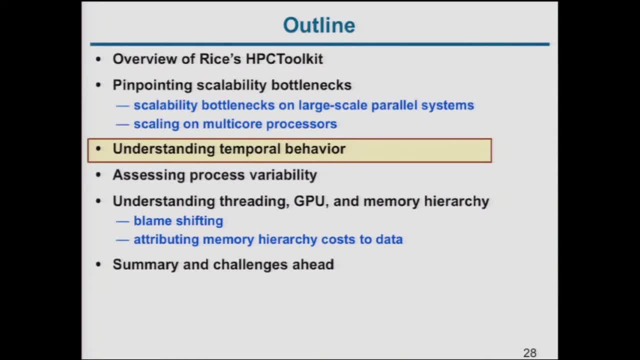 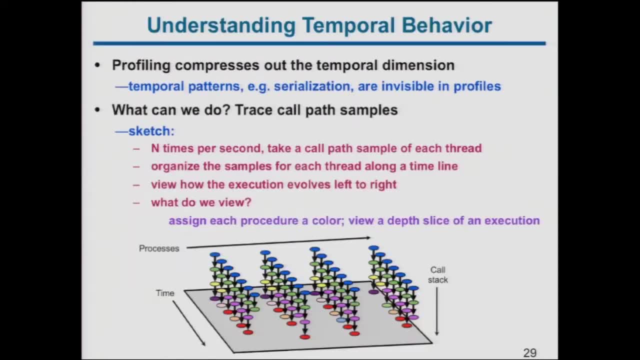 that many other tools do, where they'll add tracing in every MPI call or in the front of every function. What we're tracing over time is we're tracing samples, And so the rationale for this is that, with profiling, you're collapsing out the time dimension. 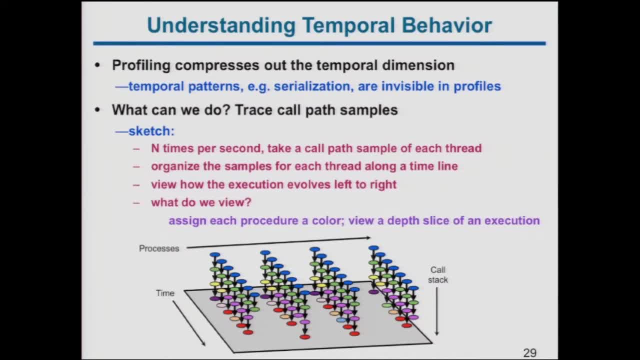 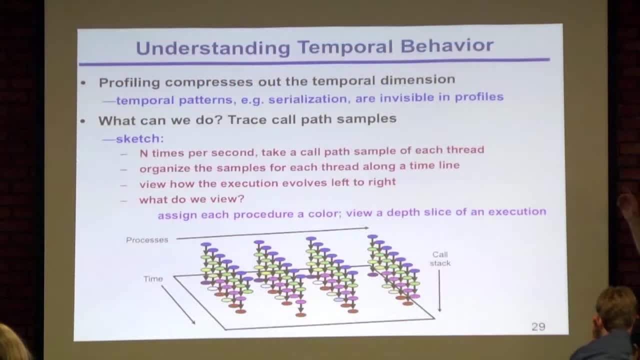 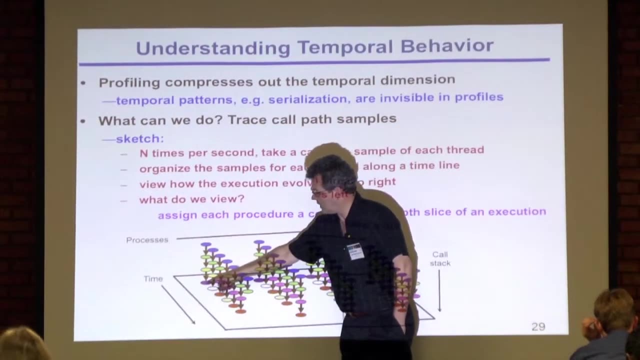 and so you may lose some information about how you ended up with a particular profile, So you might not understand how this particular profile arose. So what we do is we trace call path samples. So at any individual sample we'll get an interrupt and we'll collect a call chain for a process. 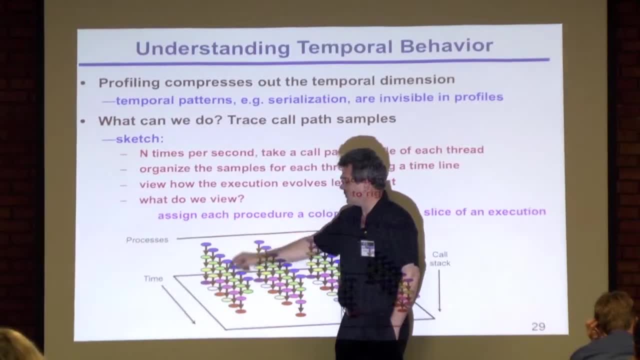 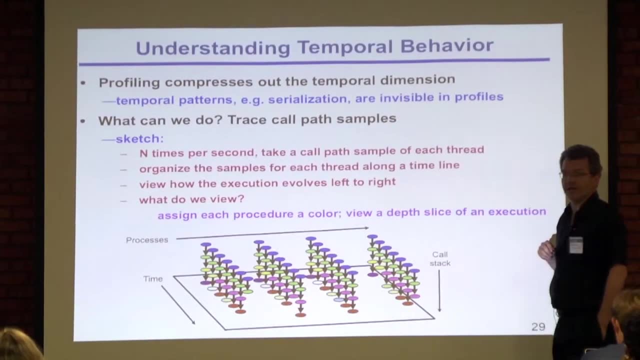 And then a next time interval will collect another call chain, And so we end up with a series of call chains for one thread and for each of the threads in the entire application, And so the way you look at this is it provides this multi-resolution view. 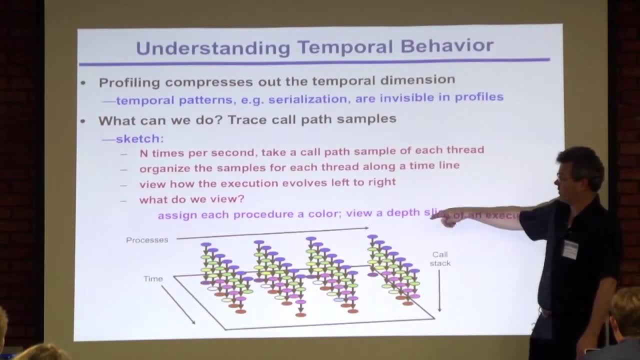 of what's going on. If we take our visibility plane and we lift it all the way up to the top, all of the dots are blue And what that means is like everybody's in main. so the dots represent a procedure and the colors represent what procedure we're in. 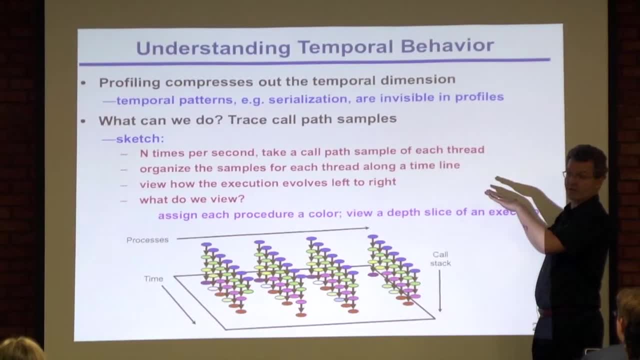 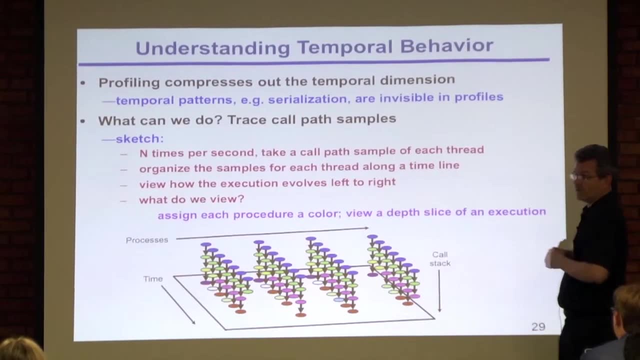 And so if I lift up this visibility plane all the way up to the top, I'll find that everybody is in main or things main, called for the entire application, And as I move the plane down I start to see things at a finer level of abstraction. 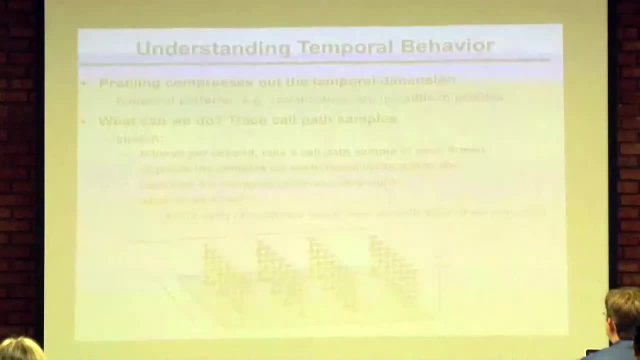 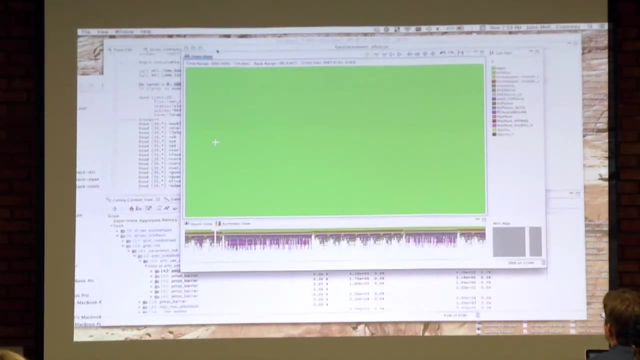 So let me show you how this works in practice. So this is an execution of PflowTran, which is a groundwater flow application developed primarily at Los Alamos. So what this is showing us is an execution of 8K cores for about 20 minutes. 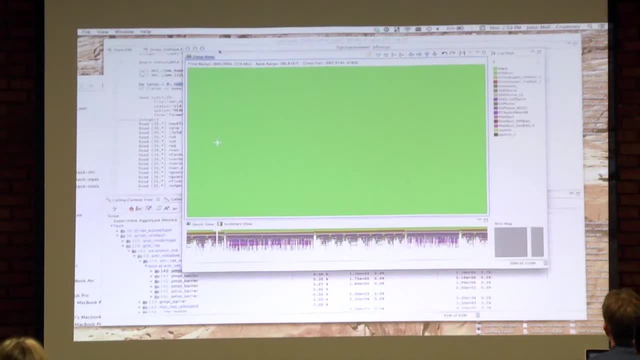 And so what we see over here is a call chain, And that call chain corresponds to this particular point in time. So that is process 4,163 at 667 seconds into the execution. Okay, And then what this is showing us on the bottom. 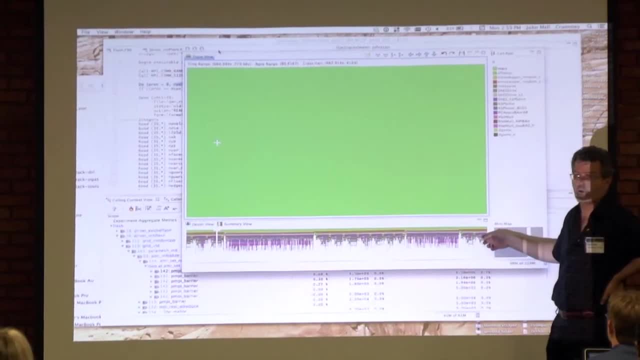 is the series of call chains over time for an individual process. Now, I don't have enough pixels here to display 8K processes, so what we're actually doing is we're sampling when we're rendering the display as well. So we look at every 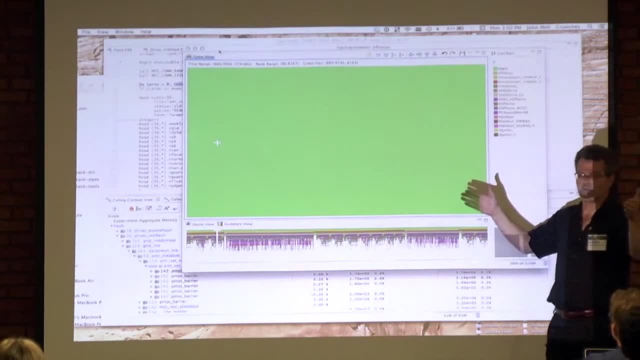 So we say we have 1,000 pixels, so We're gonna show you 1,000 points in your execution, And so this is showing that everybody is in main for the entire time. So we have threads on the vertical axis and time on the horizontal axis. 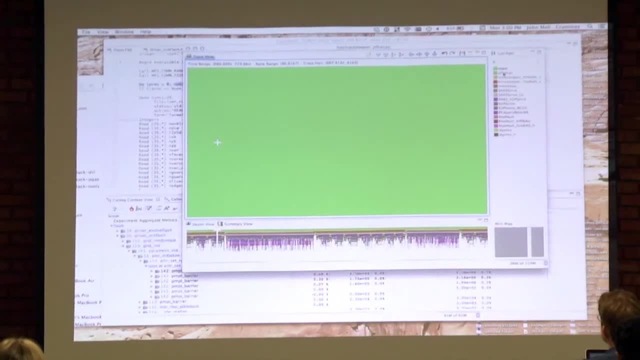 So this looks pretty uninteresting at the moment. Now, if I move down main calls PflowTran, which is the 4-Tran main, I move down another level of abstraction and Let me move out to. This is showing just a small flow. 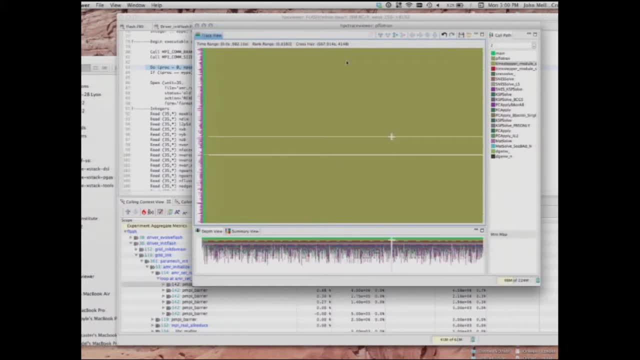 This is showing just a fraction of the execution. So if I show the whole execution, So you see that there's a little something different. There's a flex of a little different color over here during the initialization And then the rest of this is the TimeStepper module. 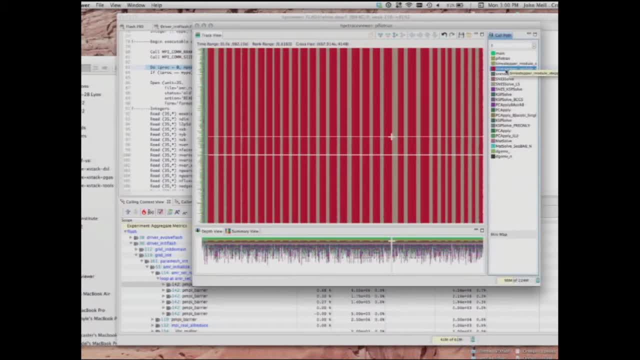 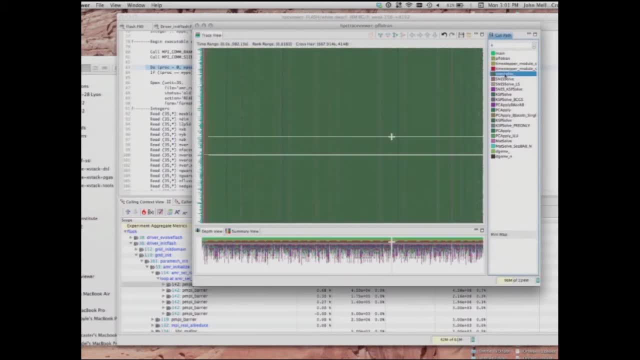 I move down one more level of abstraction and now we can see there's two colors and one represents flow simulation, the other represents transport simulation. If I move down further, we find that. well, actually both of them are calling Petsy. 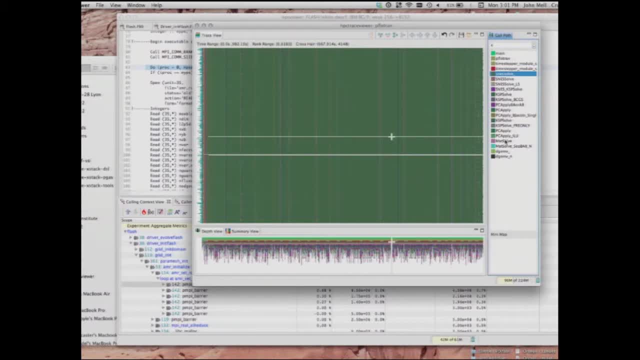 And so, in fact, we have this very long call chain that's deep down into Petsy, And so what this is showing us is how the application evolves over time. So, if I move up and just pick some small part of the execution to focus on, 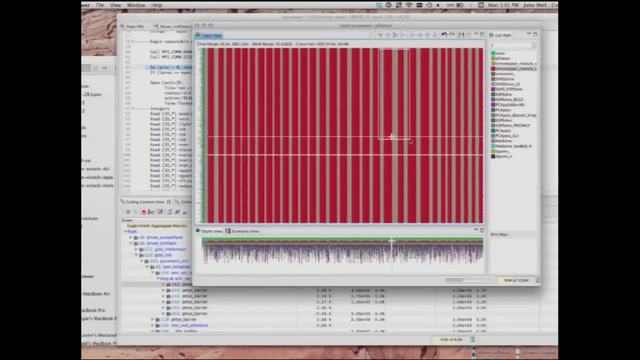 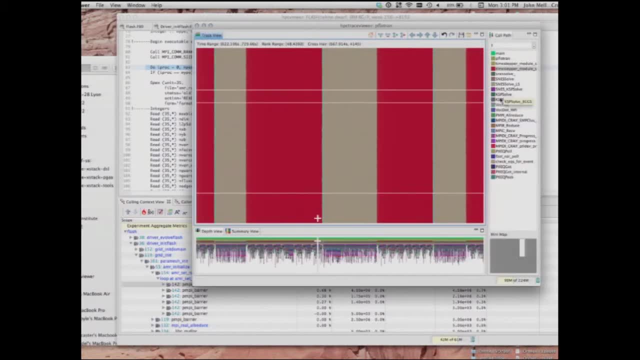 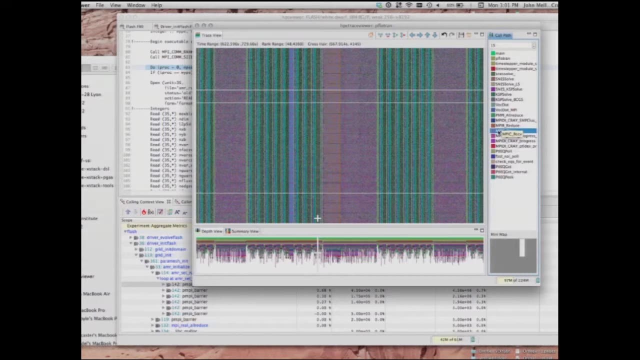 a couple of flow and transport iterations and this is about 8 gigabytes of data for these 8K cores and I'm visualizing it interactively on my laptop So I can move down a couple of levels and so you can see in fact. 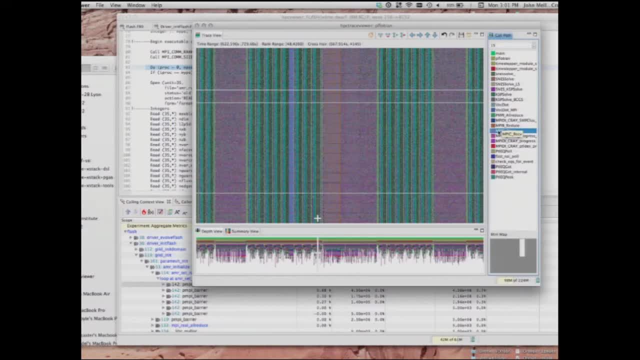 now there's even more detail of what's going on inside Petsy and you can see. so one of these was the flow and one of these was the transport, And so, even though they're both using Petsy, they're in fact using Petsy very differently. 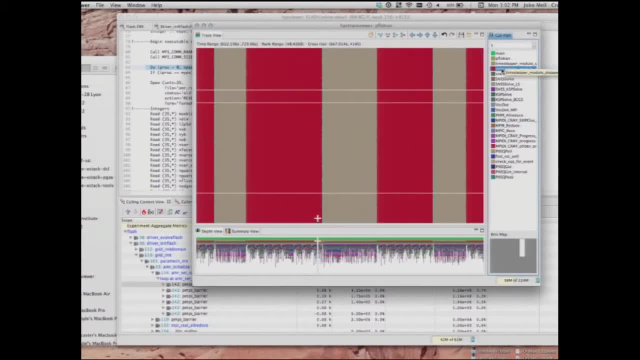 So let me just go back up to the flow and transport, And so you can see, the red is transport and this is flow, And so, even though they're both using Petsy, they're using it very differently, And then you can zoom way in. 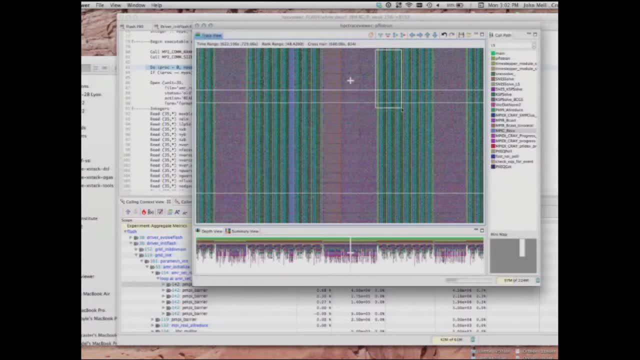 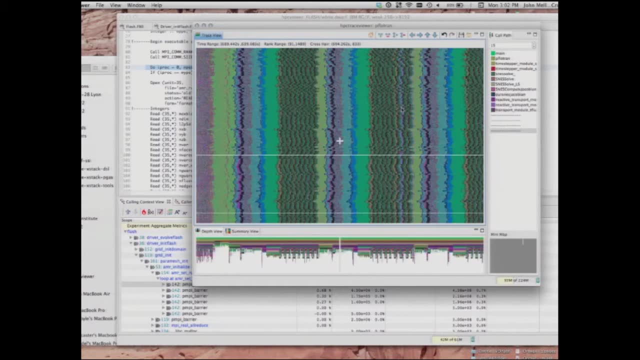 and see details about this as well, And so what we're doing is we're sampling over time, and so now we have this ability to render hierarchical views of the application over time, And so we're not doing any clock synchronization between the processes. 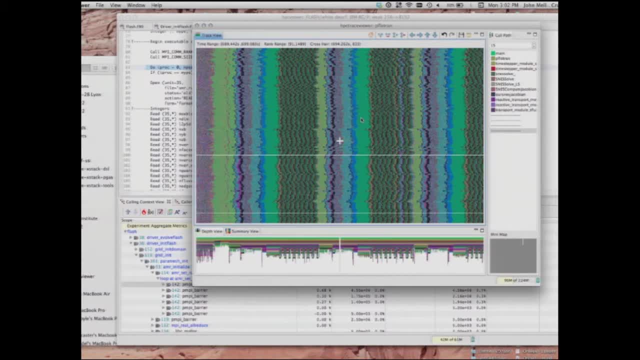 and so it's shown a little bit skewed here and that's something that we could do in a post-mortem fashion. But this whole trace was collected in about 5% overhead, And so it's because we're only tracing about 200 samples a second. 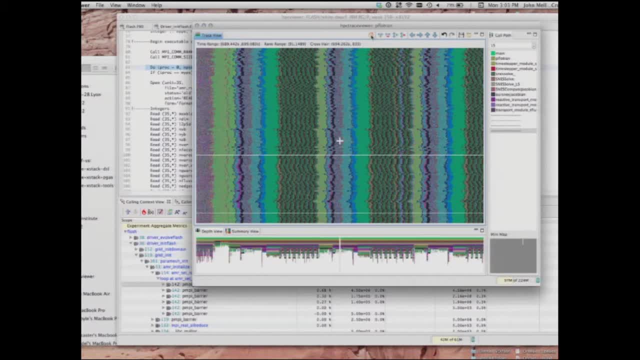 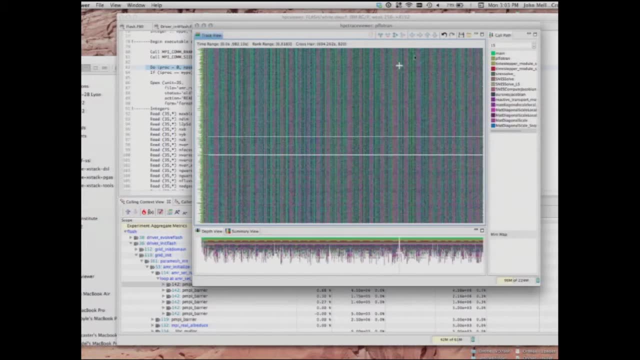 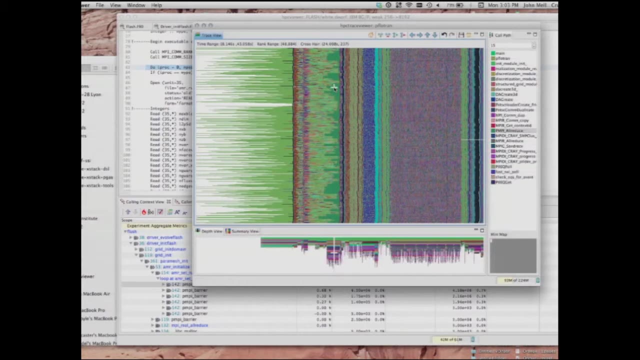 And so, but you can still see how the behavior evolves over time. So I'll just one last thing. I'm going to zoom in on the initialization phase and show you a detail of that. So what we have here, there's a call to MPC. 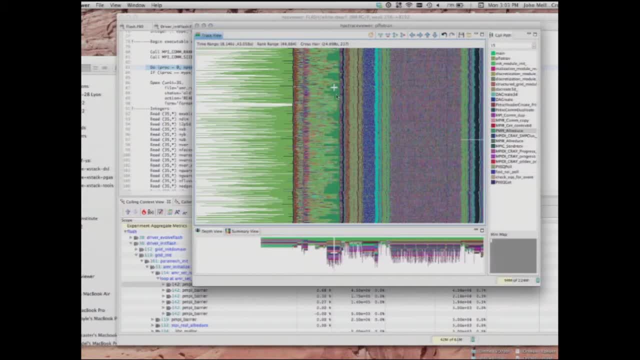 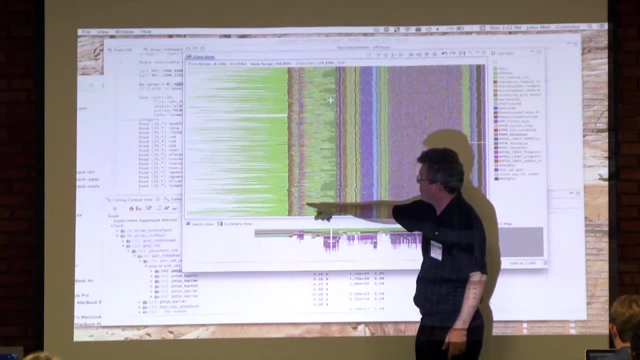 MPI all reduce, and so that's this dark green, And so what we have here is load imbalance, where nobody is finishing this phase until everybody finishes the earlier phase, And so we see these irregular splotches of this dark green And what it is. 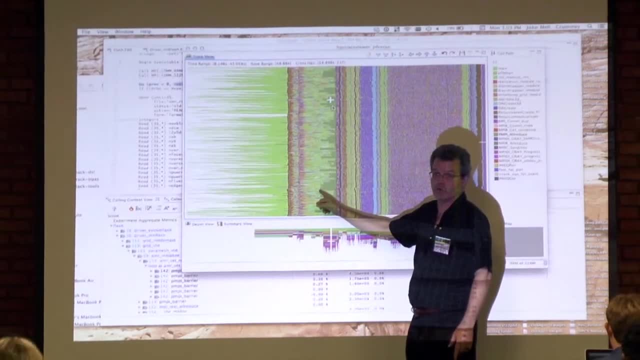 is everybody's entering a reduction. Some of them finish with the previous phase earlier, Some of them finish very late. But all of this section means that some processors are waiting around for other processors to arrive. So you can visually see load imbalance this way. 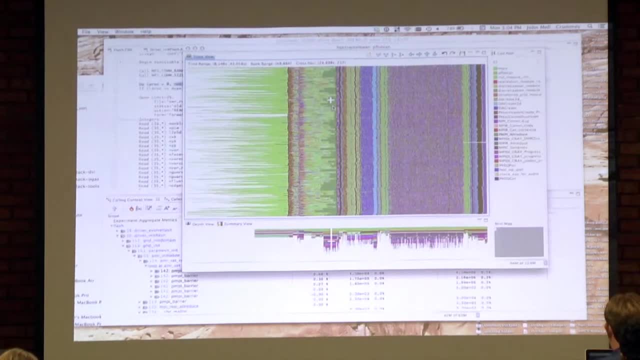 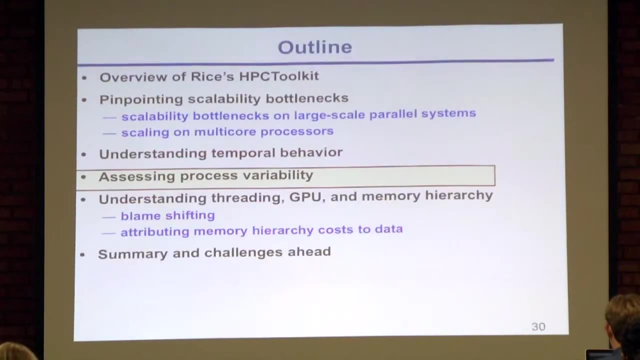 as well as you can see load imbalance in the profiles as well. Okay, Running short on time, so I'm just going to go through some of this very quickly, So to assess process variability. there are a couple of different ways you can do it. 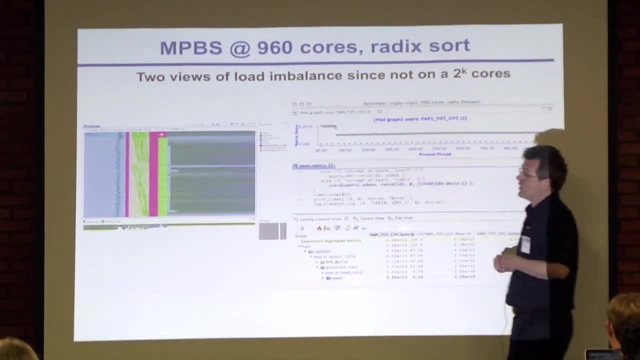 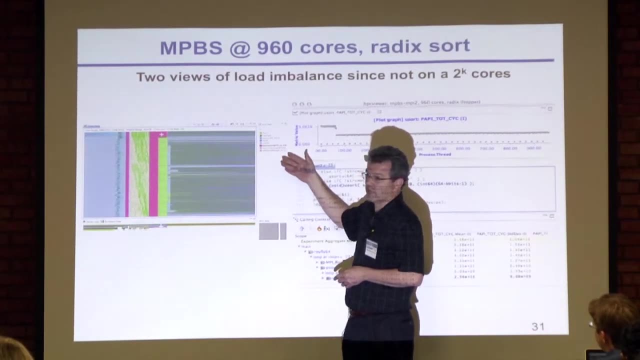 So, using the trace viewer that I just showed you, sometimes you can see it visually. This is a sorting routine. It's doing radix, sort And it's not running on a power of two processors. Some processors get a double load of work from the others. 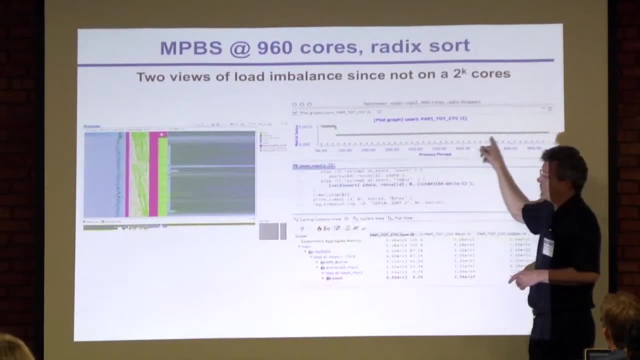 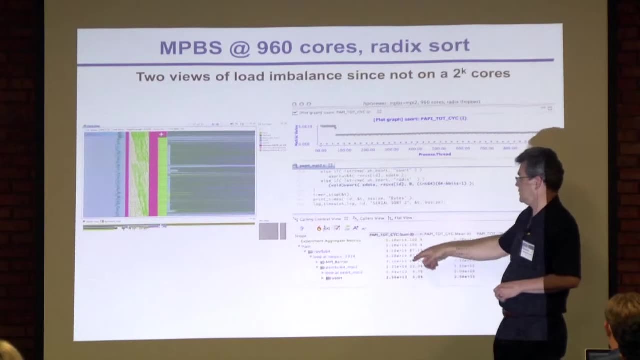 So we can see that there. We can also see it in a thread-centric view that's graphed in HPC viewer, where we can see that some threads are spending longer in the selected context. And you can't see the selection here, but it's the one at the bottom. 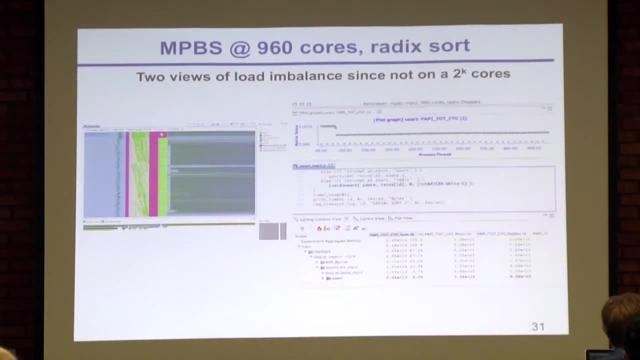 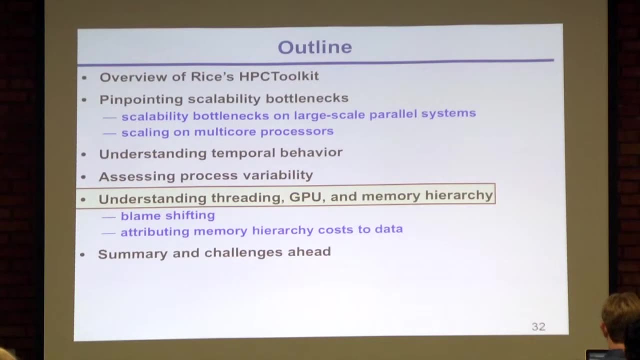 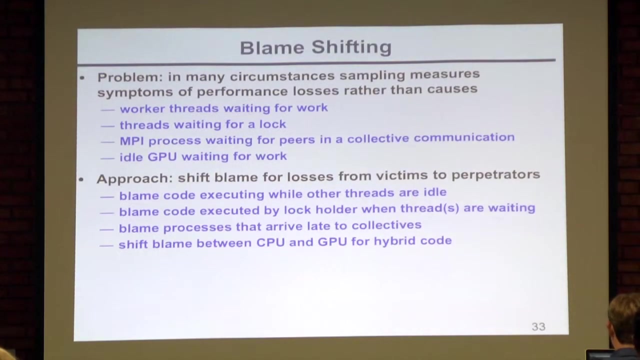 And so there's different ways where you can see load imbalance, And then also we have some support for understanding threading, GPUs and memory hierarchy, And so the problem is that often, if you're using sampling to measure something, you'll often measure symptoms. 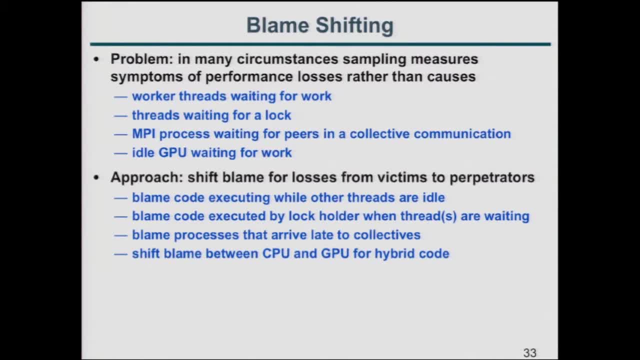 So I'll find that some thread is spending a long time waiting for a lock. Well, the waiting for a lock is a symptom. Whoever's holding the lock is the cause, And so what we'd like to do is shift the blame from the symptoms to the causes. 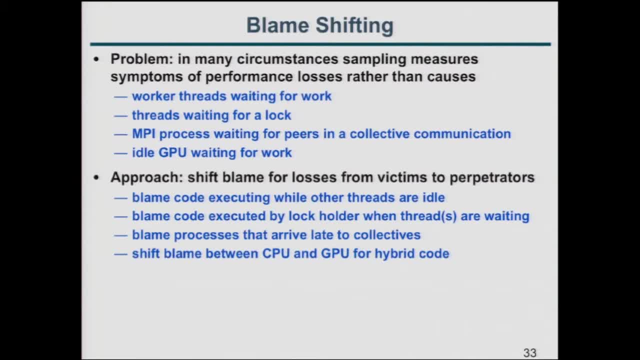 And so we want to blame code that's executing when other threads are idle, or blame code that's executed by the lock holder when threads are waiting, or blame processes that arrive late to collectives. or if the GPU is idle, we want to blame the code that's running on the CPU. 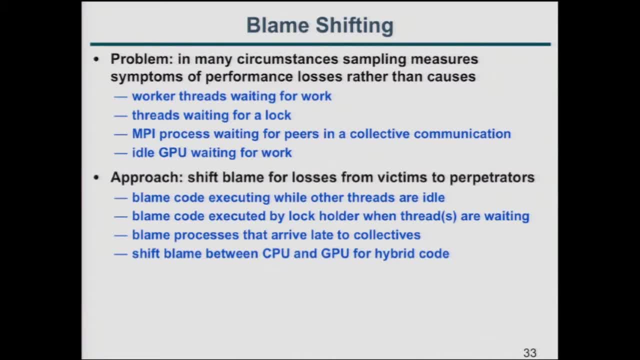 for not keeping the GPU busy. Similarly, if the CPU is idle, we might want to blame whatever kernel is running on the GPU, to say that the CPU work is not adequately overlapped. And so let's look at this. Well, the way that we do this, 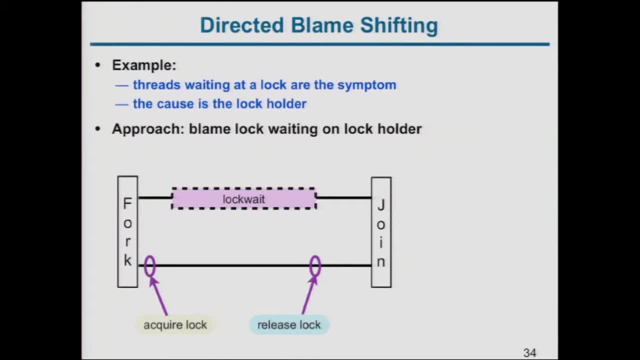 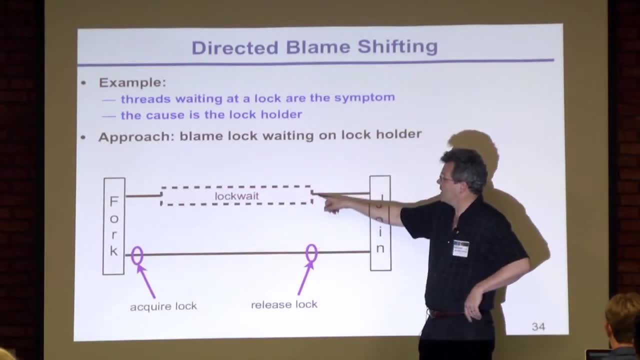 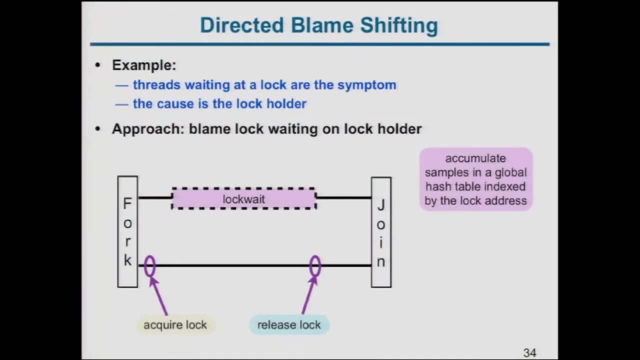 we have this general technique that we call blame shifting. And so for locks. suppose one thread acquires a lock and then releases a lock In the meantime some other thread is waiting for it. Well, what we do is we accumulate samples in a global hash table. 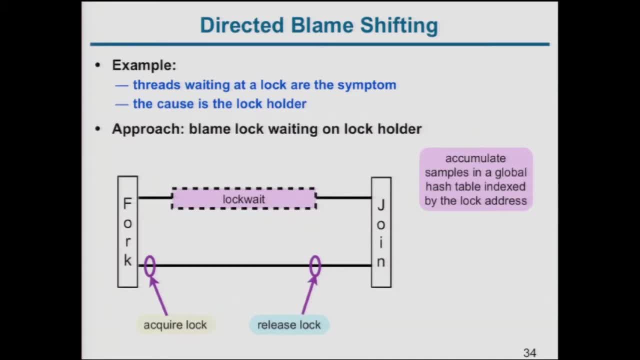 that's indexed by the lock address. And then, upon the release, the transfer, the lock holder says: has anybody been waiting for this lock? And they check in this hash table they find out how much cost has been attributed to the lock. 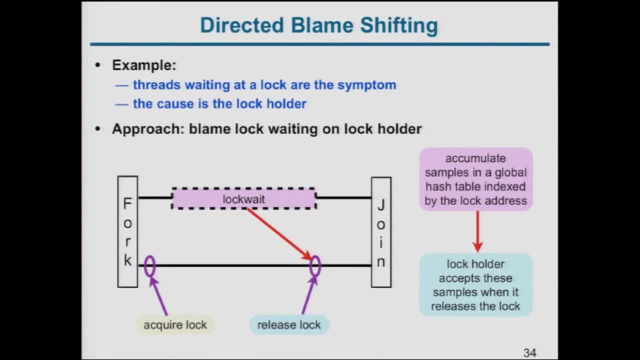 and they say it's my bad, And they'll attribute it to the lock release. and so you know, at the point that they release the lock, that they held up a lot of or a little of of processors keeping them from working. 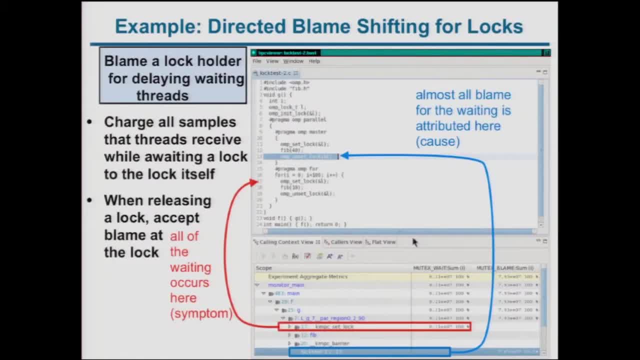 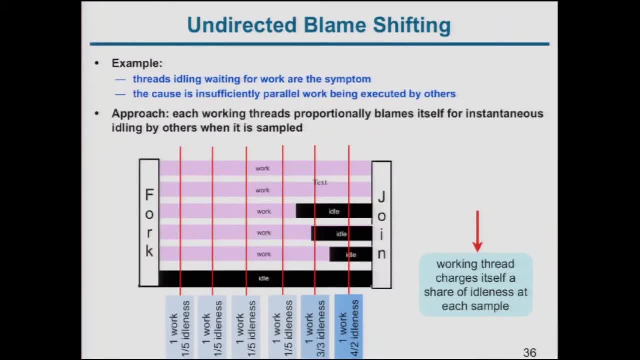 So that's directed blame shifting. There's also something called, so this is just an example that shows how it works for locks, and I'm not going to go into this since I'm sort of short on time. So let me explain undirected blame shifting. 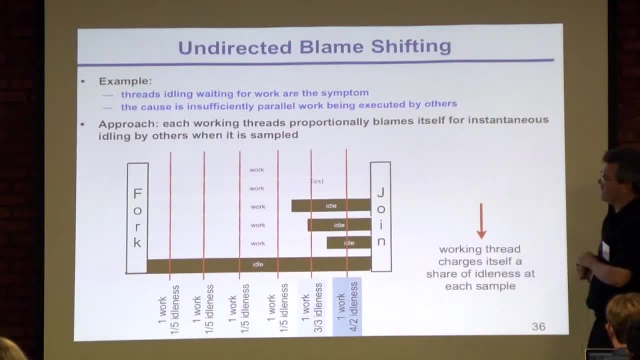 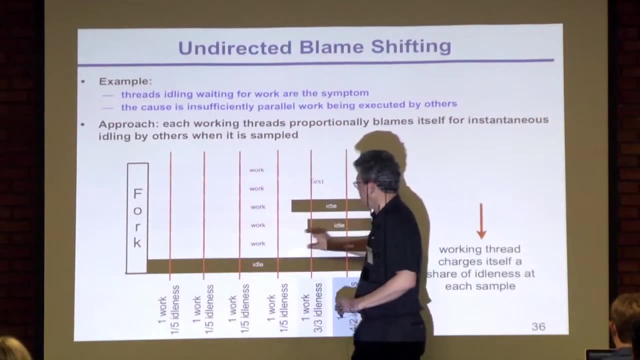 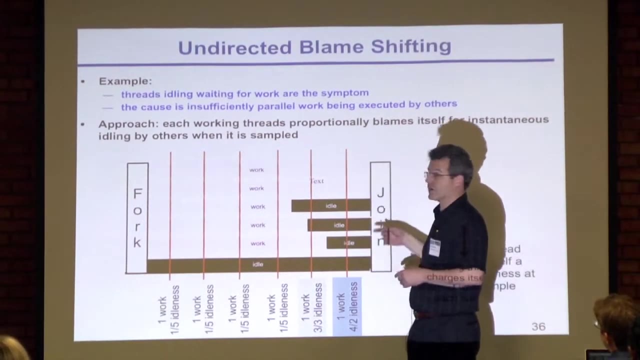 So here consider, we have a bunch of threads and I really hate that the color washed out. So this had light purple bars across here, and so the black was for idle and every other thread was working, except where shown in the black. 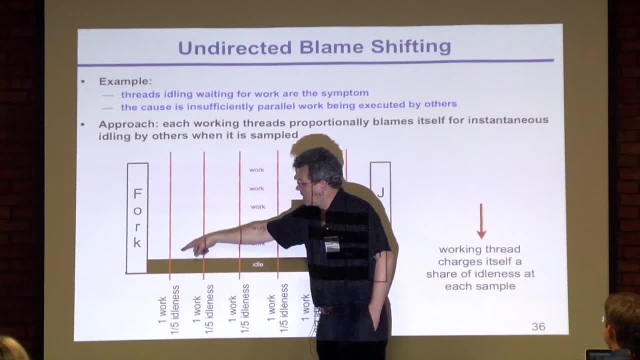 And so what would happen is, if we took a sample here, all of the threads would be working except for one, and so each thread would say I get one unit of work, and since there were five threads, they would say I'm going to charge myself. 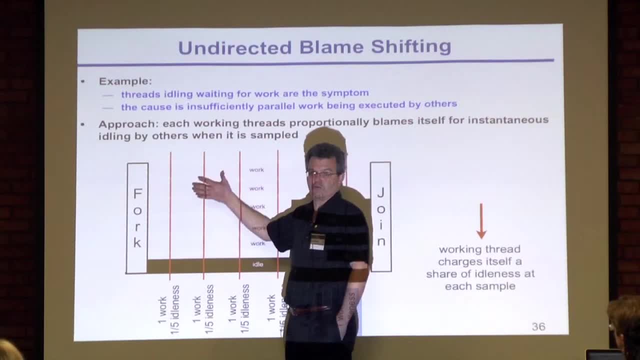 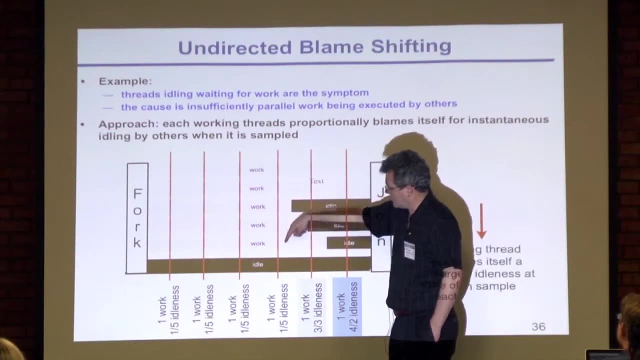 one-fifth of the idleness. There's one thread that's idle. there's five of us that are working. I'll take one-fifth of the blame for my sample And then they keep doing that all the way through here as their sample. there's only one thread idle. 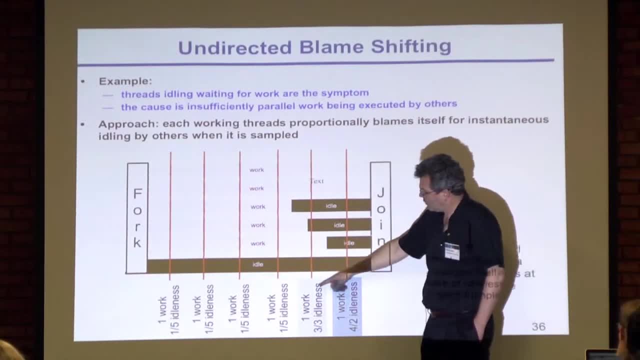 and so we keep doing the same thing, and then, as more threads become idle here, we find that at this point in time that three threads are idle and there are three threads working, and so we get one sample of work and then three idle threads. 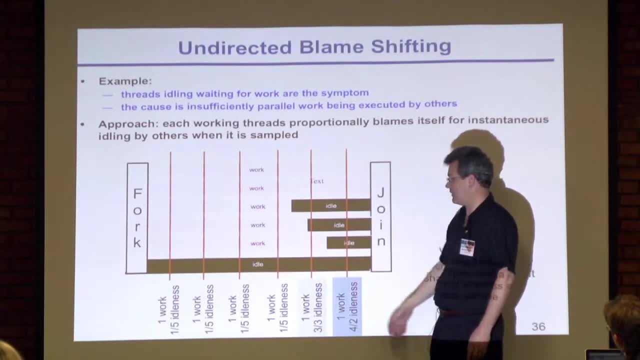 we divide up the blame for it, so we get three-thirds- is one unit of idleness, and then when more threads are idle. so what we're doing here is by just maintaining a count that says how many threads are idle and how many threads are working. 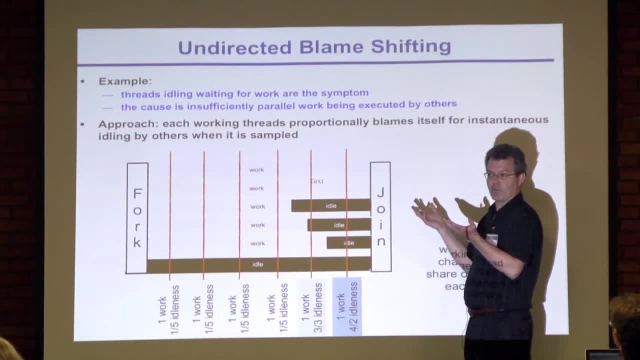 then, when a thread is working, he says: is there any idleness out there? Let me take my part of the blame. And so what that's doing is it's shifting the blame from the threads that are sitting idle to what code is executing while the threads are idle. 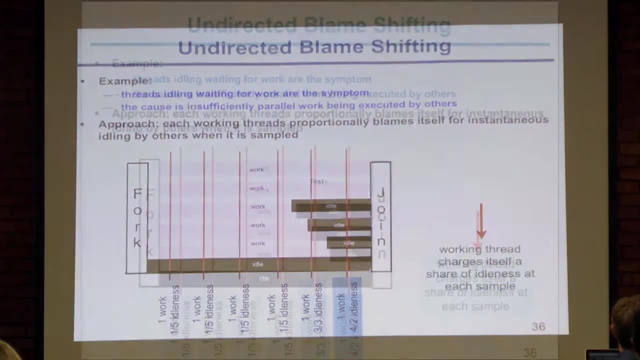 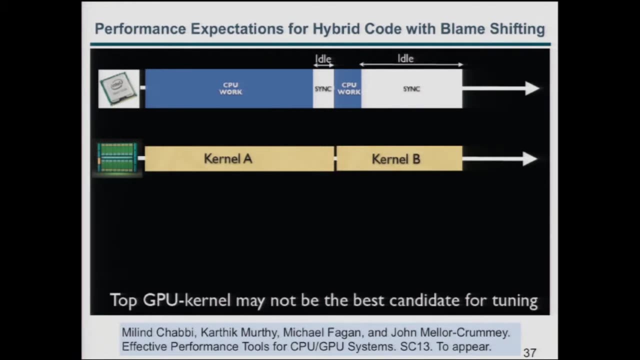 and we can show that in the source code-oriented view. Okay, So we do the same sort of thing for GPUs, and I'm not going to get a chance to go into the details, but the important thing here is that it may be the case. 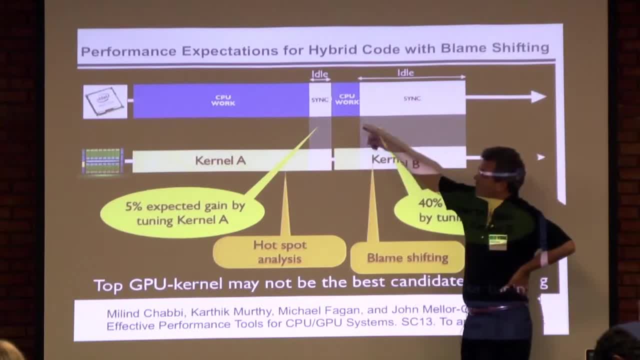 that for the longest kernel, this kernel might be overlapped with a lot of CPU work and there might be some shorter kernel where the CPU is sitting idle And so if you shorten this kernel then you can shorten the whole execution. If you shorten this kernel. 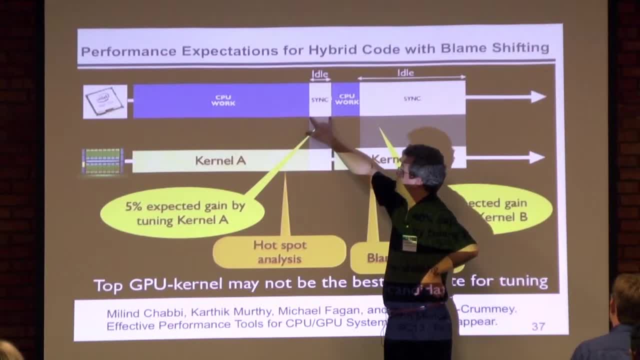 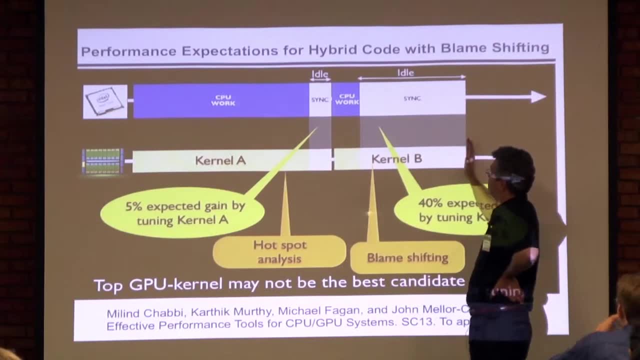 the only amount of improvement you'll get is the synchronization time. So if I make this kernel any shorter, then it's not going to help, Whereas this kernel I can bring it all the way back to here and that'll shorten my execution time. 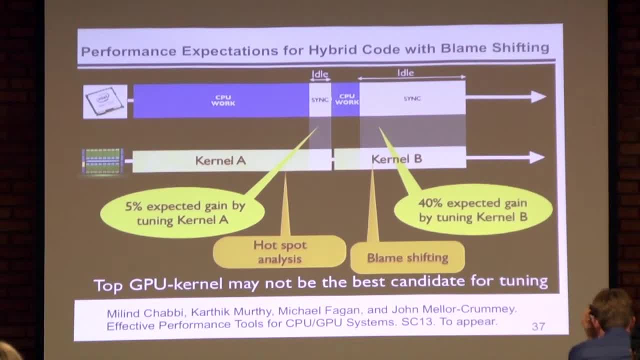 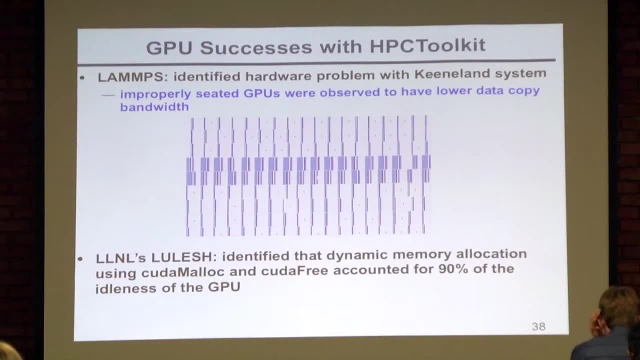 And so what we can do is tell you you should be tuning your code. So we've used both our trace-based tools and our blame-shifting-based tools to identify problems. on both Keeneland and on Titan, We identified a hardware problem. 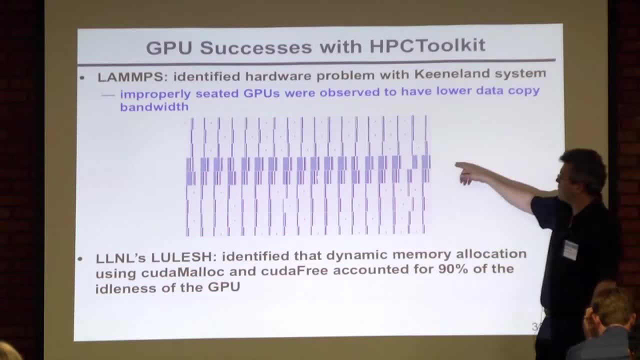 This was showing where GPUs were not seeded properly, and so the data transfers on certain nodes were taking longer, and so this actually corresponds to time for a CUDA mem copy, and so it turned out that the border records weren't set right, And so there was a hardware problem that our tool showed. 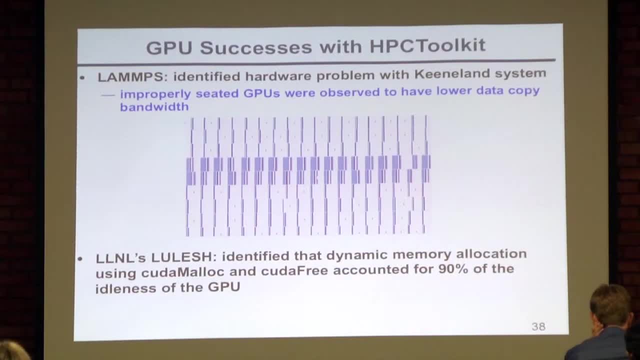 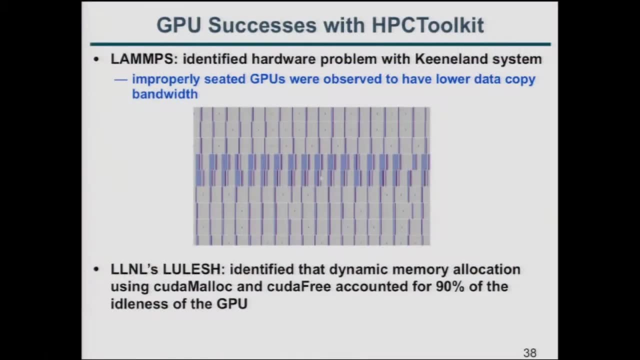 And then, using the blame-shifting, we found that dynamic memory allocation was taking a significant fraction of the execution time on Lawrence Livermore's LULESH code, And so what we found was that the GPU was idle when you were using CUDA malloc. 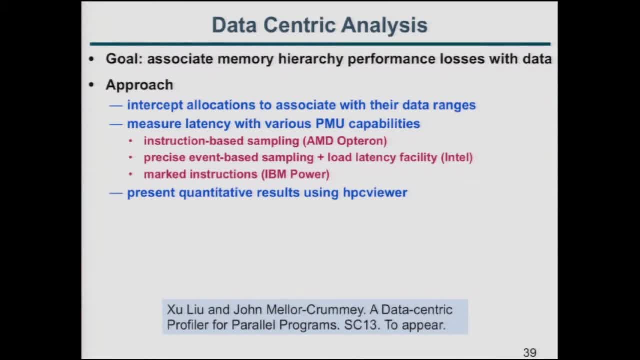 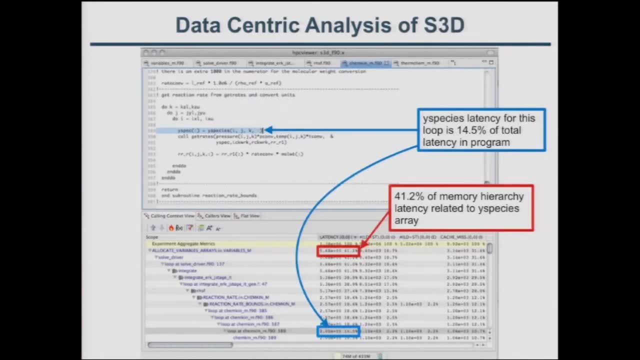 And we also have a way of attributing costs back to data, And so this is using the hardware counters, and what we can do is say that a certain- Here's a fraction of the latency that's attributed to a particular variable, and then we can attribute it not just to the variable. 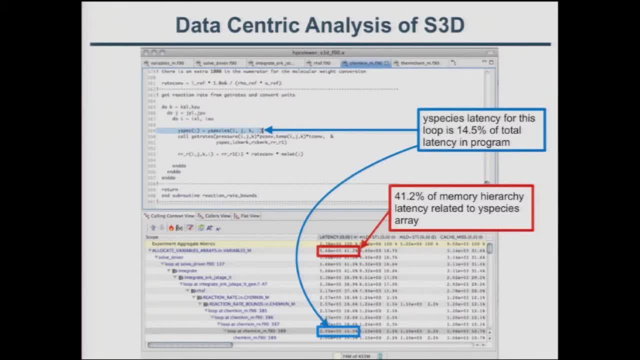 but also to individual source code lines that are touching the variable. Now this is a really useful capability. You can't use it on very many machines. It turns out that the kernel capabilities that are needed to get this data out of the hardware counters are hard to come by. 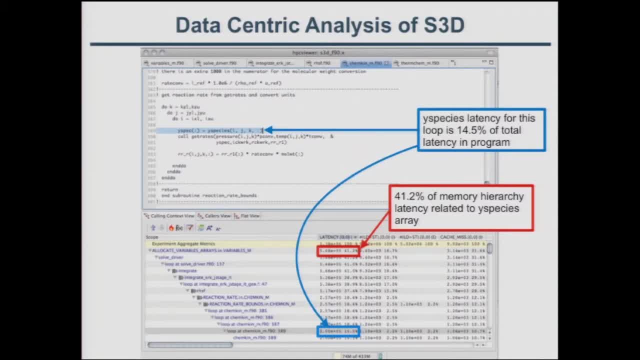 They were in Linux kernels through 2.6.30, and now they're coming back in 3.10, and none of the machines you're working with have anything like that. And so sorry you can't get this data on Titan.